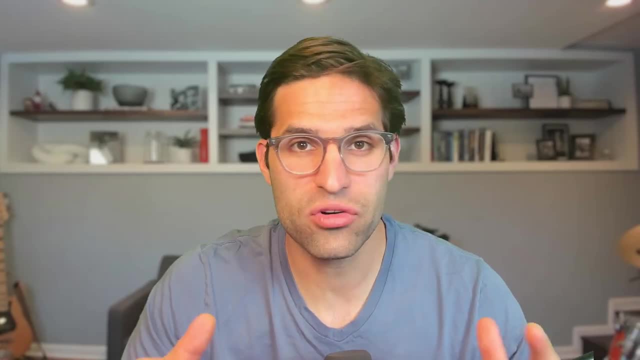 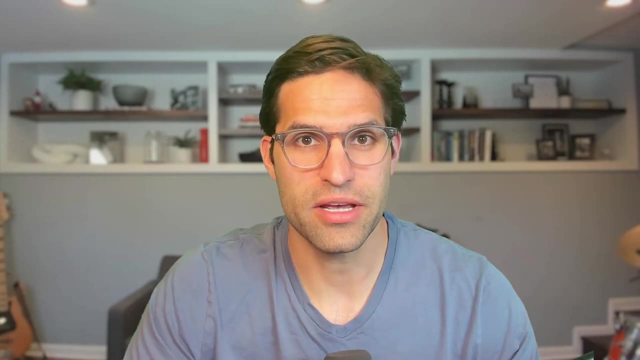 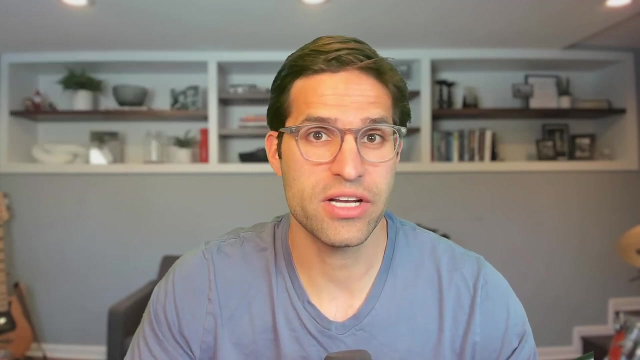 used and when to use them. And finally, we're going to apply the correct cross validation to the first model that we showed and show how we can actually evaluate it in a proper manner. If you enjoyed this video, please consider liking and subscribing. You can also check me out on Twitch, where I stream. 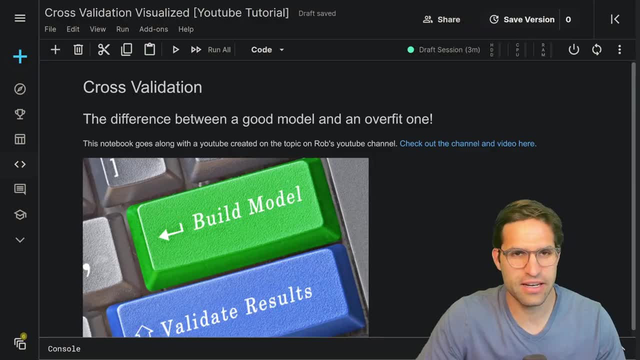 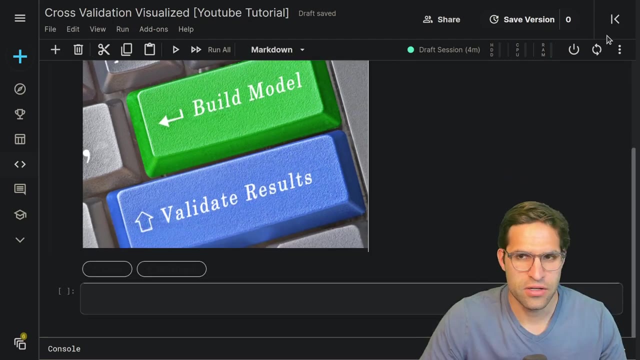 All right, let's get into it. All right, so here we are in a Kaggle notebook. Now, the nice thing about this notebook is I'll link it in the description below and you'll be able to click that link and come into the same data set and go through the code later if you want to. So 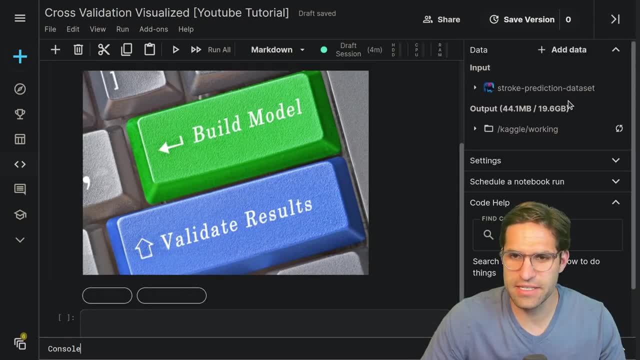 before we get too far here, I want to show you. I've added a data set called the stroke prediction data set. We're going to be using this as an example for showing why cross validation is important And basically this is our plan for this video. We're going to show an example where 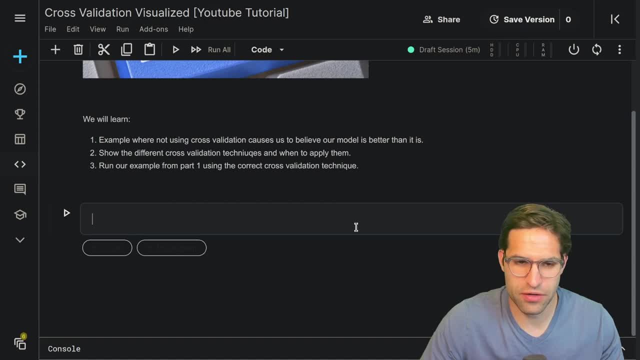 cross validation is important. step through all the different cross validation techniques which I commonly use and then run our example with proper cross validation to show how that actually works in practice. We're going to do a handful of imports here, So these imports we import most. 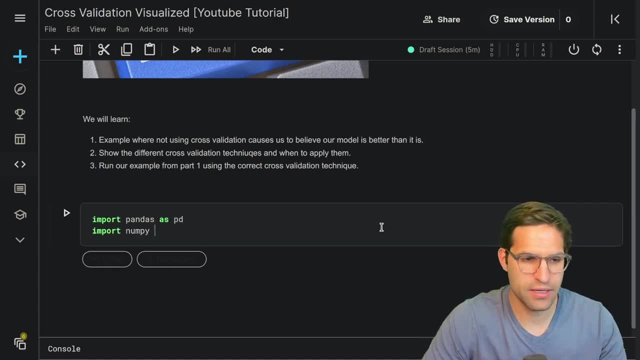 of the time. So import paint Pandas, Import numpy, Import matplotlib. Now for our model. we're going to import lightgbm And you don't need to know that much about that model, other than the fact that it's a machine learning model And without proper cross validation, we're going to see that it'll. 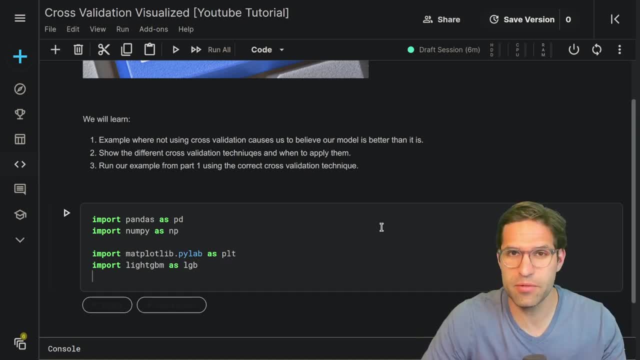 over fit to our data. But this could really be any type of machine learning model, as- and we're just using this as our example- Now we're going to import some metrics from sklearn. sklearn We're going to import accuracy and the area under the curve score. 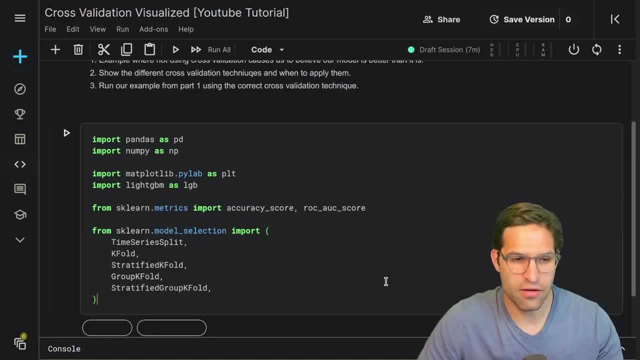 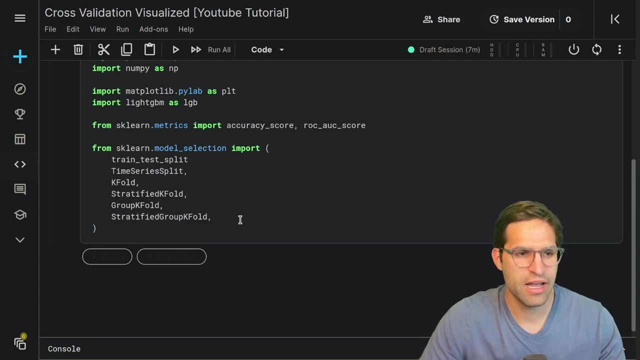 And now we're also going to import here a bunch of model selection techniques from sklearn And let's also import train test split. But these are basically in sklearn, which is a very powerful machine learning library. They've already built in a lot of these cross validation techniques for us. 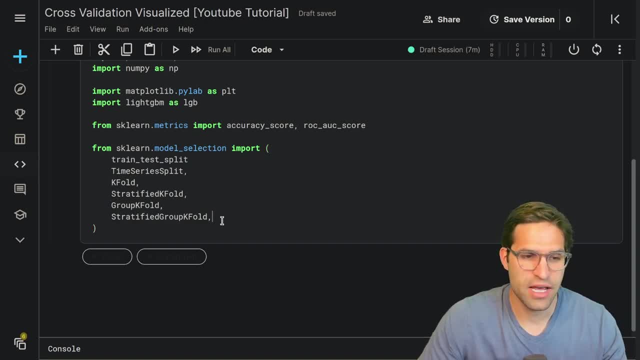 So all we have to do is use the predefined objects and apply it to our data set to get the cross validation working, And we're going to import all those. at the start here, Make sure i do a comma. Okay, so i already said we imported a data set, but a little bit of information about this data set. 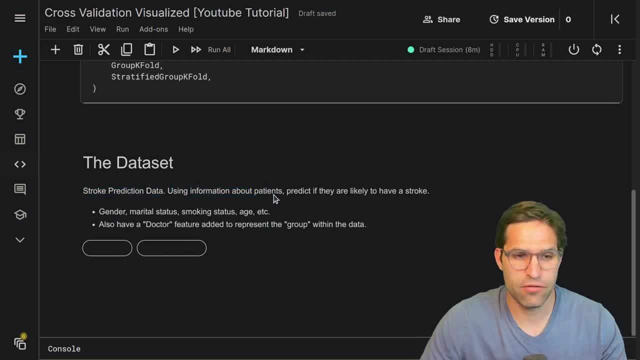 It's the stroke prediction data set. It's using information about patients to predict how likely they are to have a stroke, And you can imagine this being important for medical fields. We We're also adding in a column that we're making that's just fictitious. that'll represent the doctor that gathered the data. 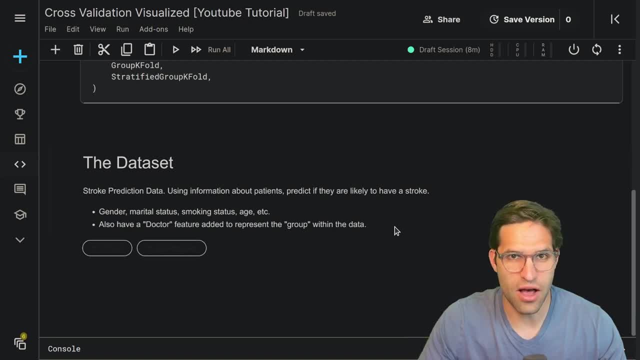 And the reason why we want to add that to the data set is because often when you're doing cross-validation, it's important to group your different your data sets by anything that's common amongst them, And we'll show that later And in this example it'll be something like the doctor. 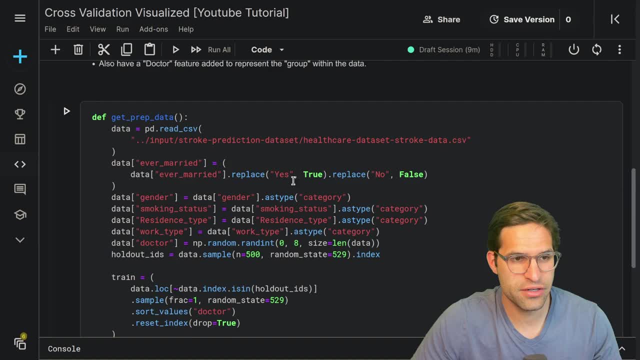 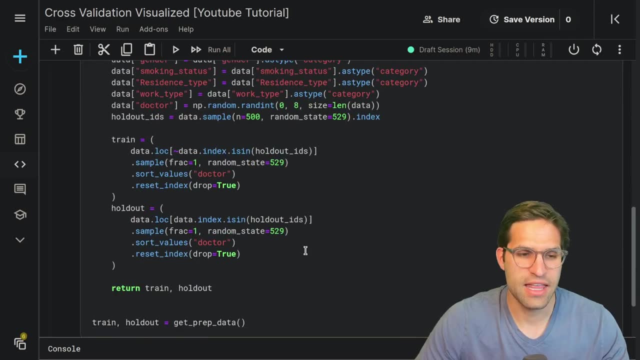 Now I've created this, this function, beforehand. All this really does is reads in our data with pandas, It sets the format of the data and then it does a simple split where we take some of the data and we make it our holdout set. 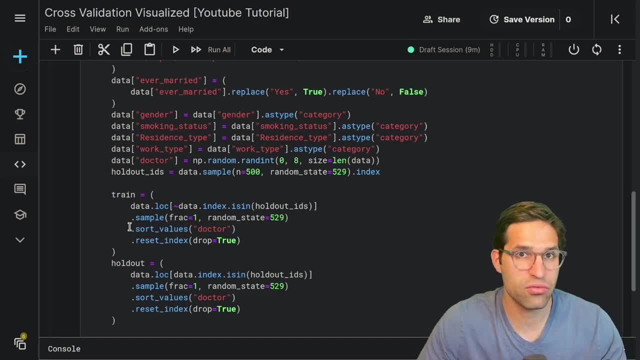 So imagine this being like data in the future that we plan to run our model on. And then we have our training set, which is a bunch of label data that we have for this data set that we'll want to train our Machine learning model on. 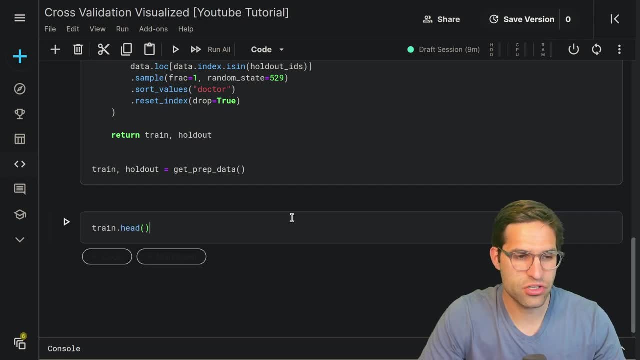 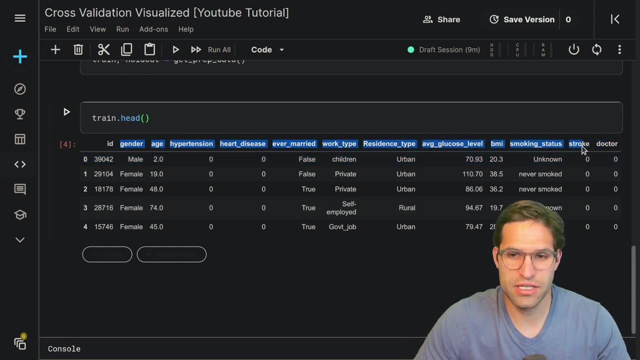 So if we run this function, you can see that I have this train data set with a bunch of different features about each patient, And then you can see here on the right side the stroke column is either a one or a zero And that's what we're trying to predict for the data set. 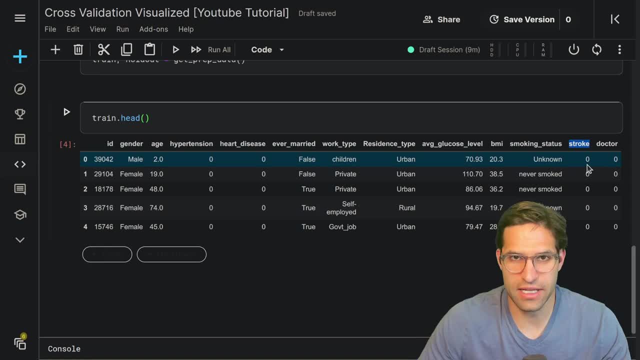 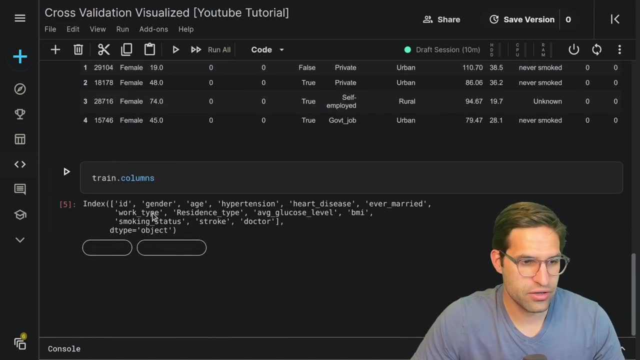 If the patient had a stroke or not, or was high likelihood of having a stroke or not. Now, of all these train columns, I can show you here that most of them will be our features, and then we will want stroke to be our target. 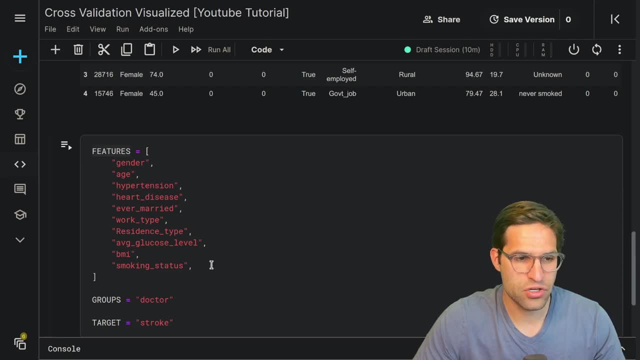 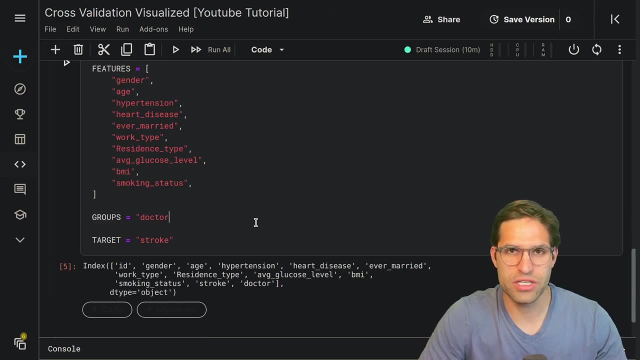 So I'm just going to make variables called features. with each of these features that we have in our data set, We're also going to name something called groups, which is the doctor, That's the different group we're in, And then target equals stroke. 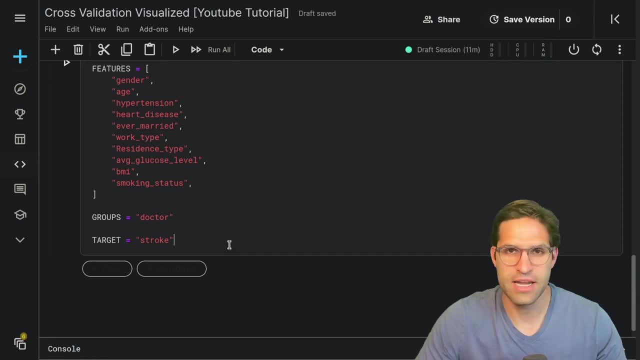 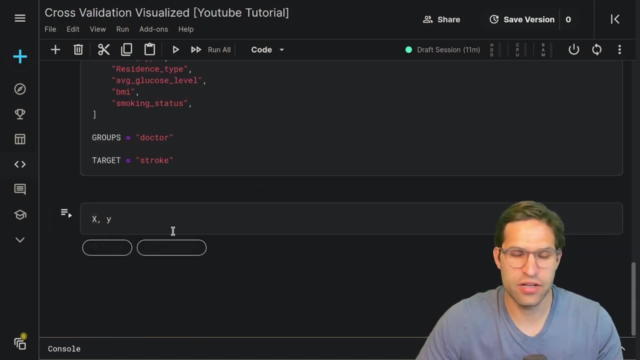 That's the thing that we're trying to predict out of this data set. Now, very commonly in machine learning, you'll have an X And a Y variable. X is just the features in your data set and Y will represent the target that you're trying to predict. 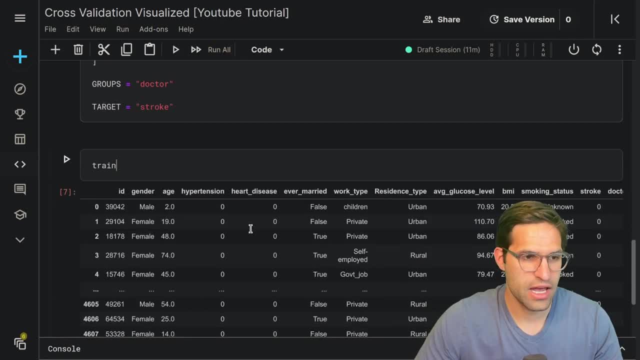 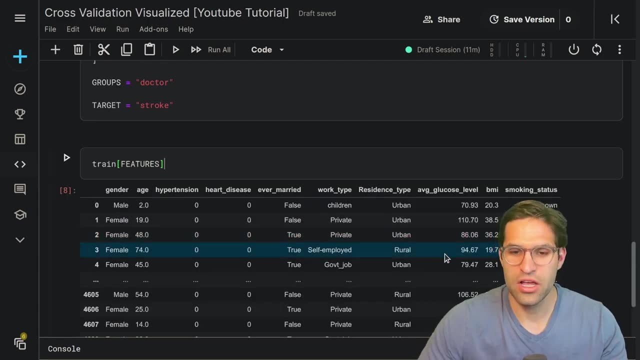 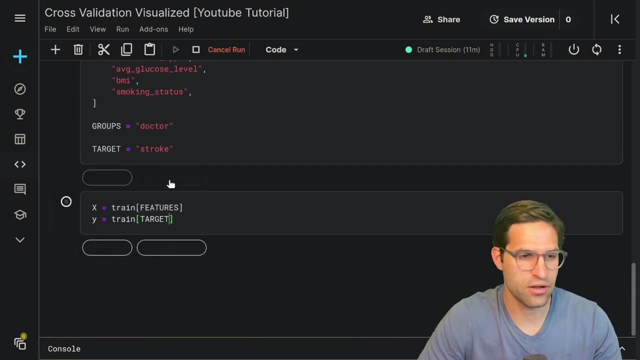 So let's take this training data frame that we have and let's make an X and Y out of it, And we'll do that by getting the features as our X And then. so let's call this: X and Y will be our target, our target column. 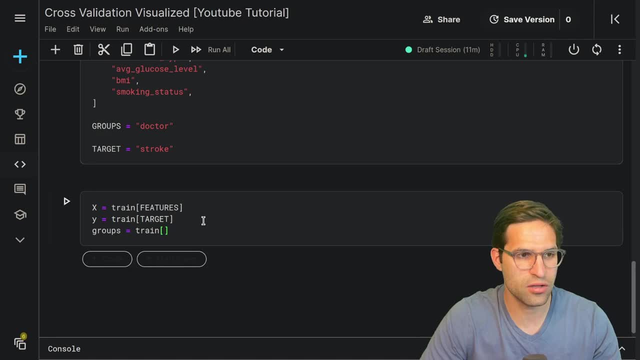 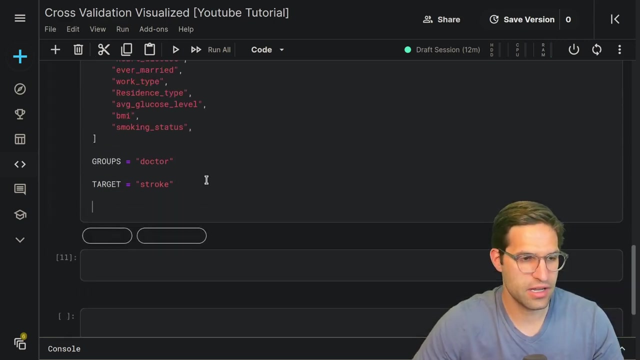 And then our groups will just be this group Group column which will represent which doctor pull gathered the data for that given patient. Let's go ahead and wrap this in a function so we can pull this with our training data set whenever we need it. 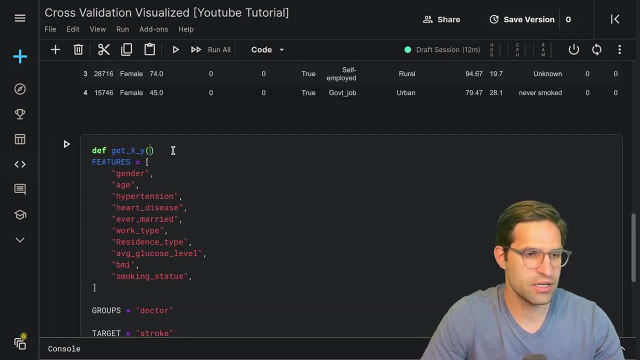 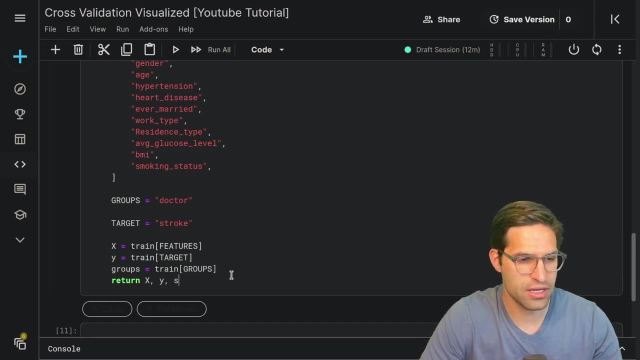 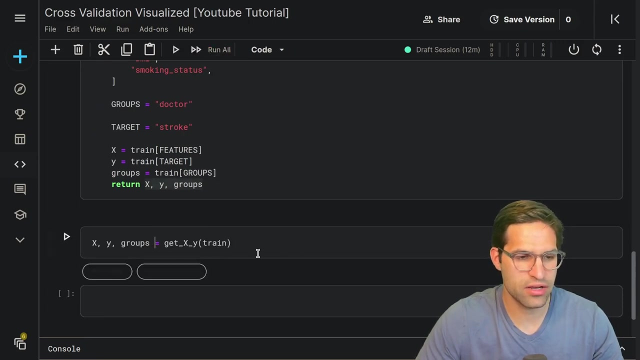 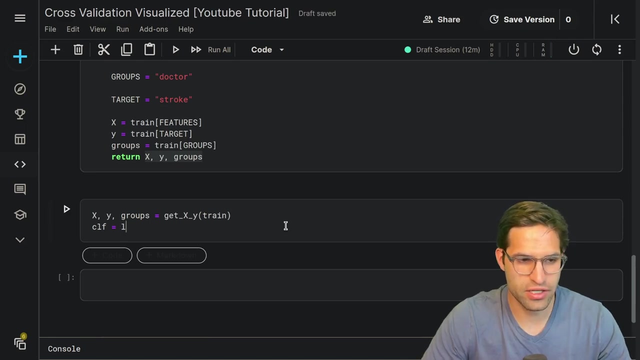 Let's define a function called get X- Y and we'll give it our training data and it will return X, Y and groups. Now, if we Run this function, we now have our X, Y and groups data and we're going to go ahead here, be super excited about this data set, want to make the best machine learning model we can, and let's just create a classifier for this using light GBM. 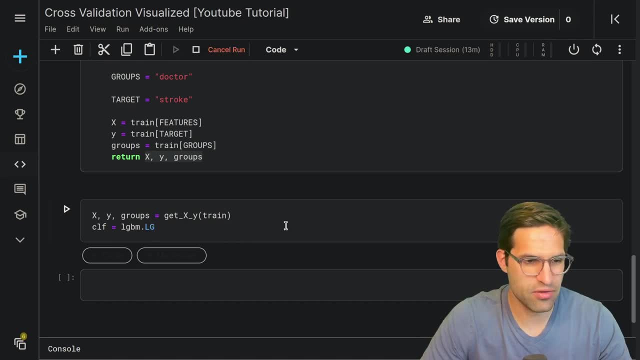 So this is just that machine learning library. That's a gradient boosted tree. It's a very common, very powerful machine learning model. We're going to set one parameter here, That's the number of estimators, and that's our model. Then we're going to call fit on our training data with first the features and then the target and looky here. 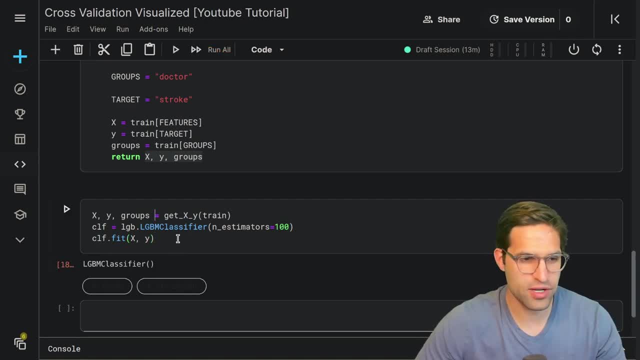 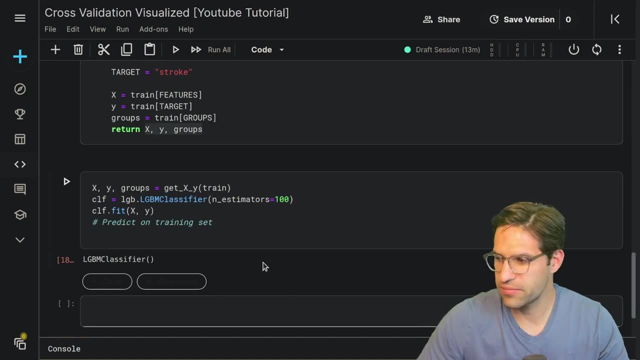 We've trained our model. It's a trained model and now we actually want to predict on our training set, just to see what the predictions look like. so we can do that pretty Simply with a classifier. we can do predict, which will give us just a one or a zero, and that it will call that pred and then we'll call pred prob, which is with a classifier. 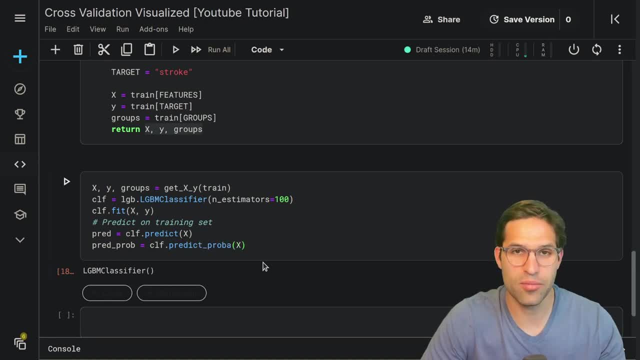 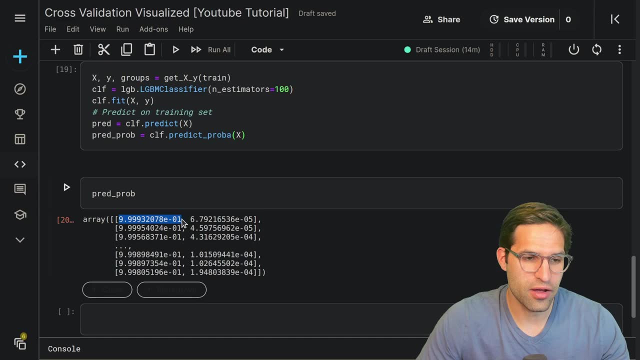 You can do predict proba, which will predict the probabilities, instead of just a binary one zero value. Pred proba actually gives us an array with both the positive and negative class predictions, and we just want the predictions for the positive class, So we'll just 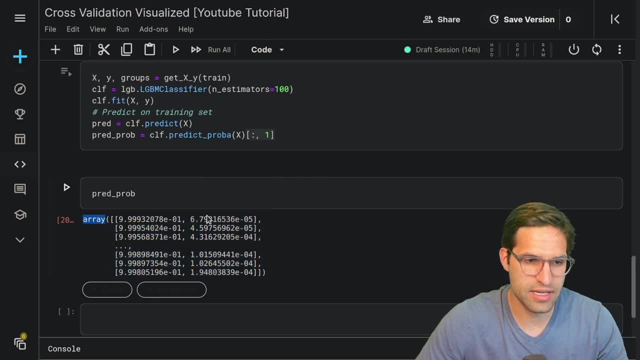 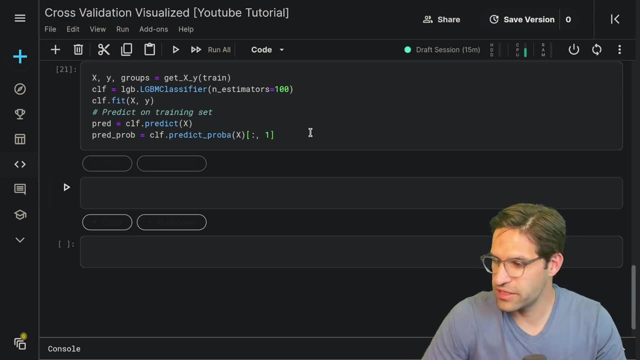 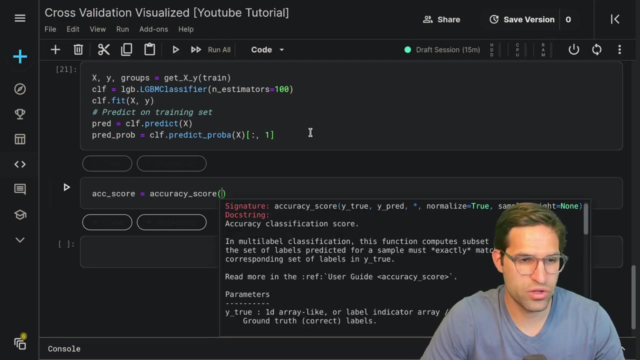 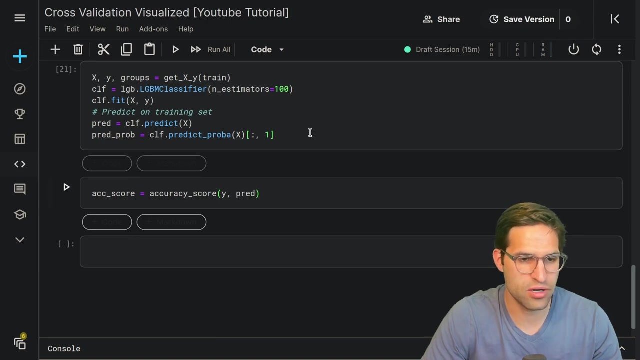 We'll add this to the end, which will just pull out the second predictions in each of these. All right, we're doing pretty good. so we've trained a model. All we have to do is score how well it did. So let's get the accuracy score- and this is a function from SK learn, where we just give the true values, which is why, and then our predictions, which is pred, and let's go ahead and get the AUC score- AUC. 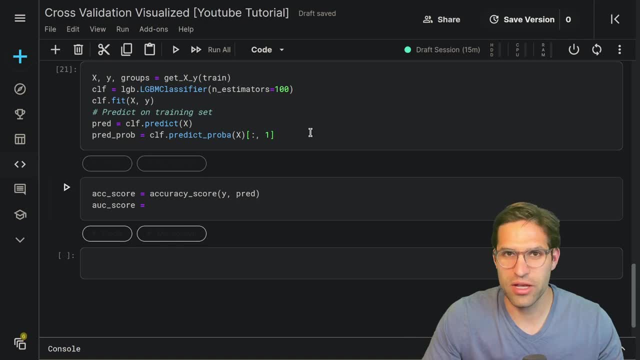 Or Area under the curve is just another way to evaluate binary predictions, but you actually feed it in the probabilities. so this is a better way than accuracy. that we'll see here in a second why it's better to use in this case. So, but we'll also feed this in. but we're going to feed in the pred prob. 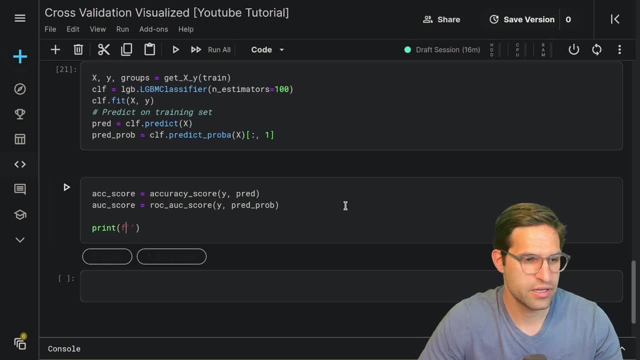 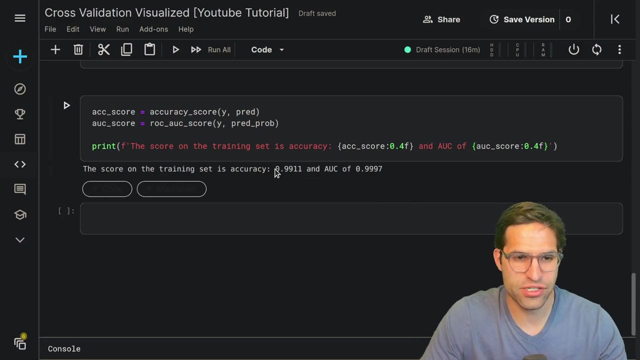 Let's go ahead and print these out. So we're going to print the score on the training set is Accuracy of X score and AUC of AUC score, and we're just going to do it to the 4th digit. Oh, my goodness, our model has an accuracy of 0.99 or 99% in AUC of 0.999.. 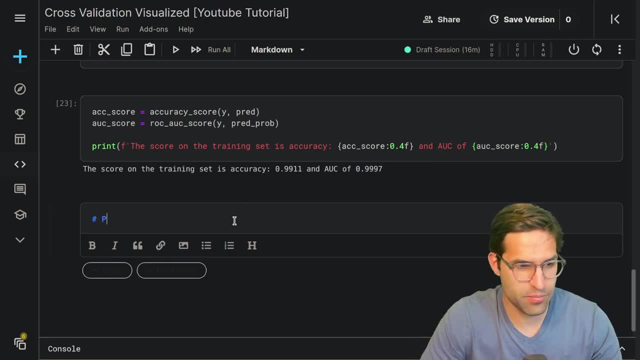 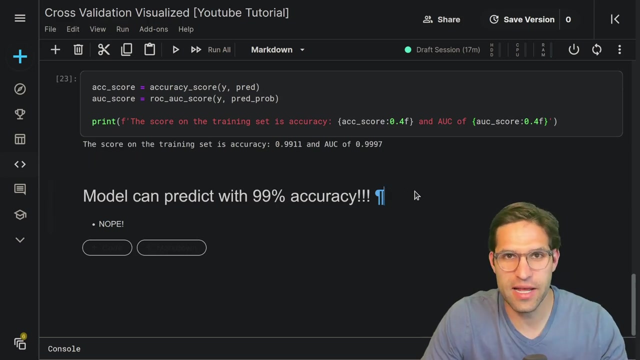 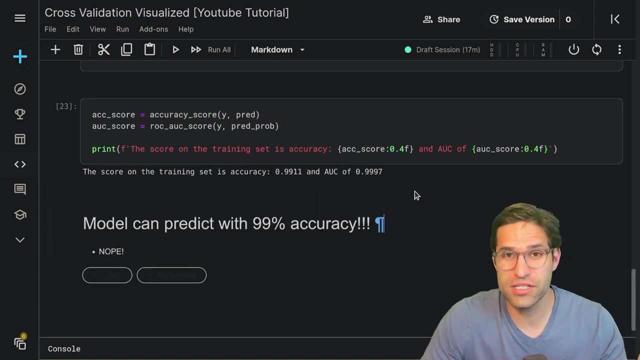 This is a really good model. All right, let's publish a paper. Model can predict With 100- wait, no, 99%- accuracy, but let's get this published. It's awesome. That's not that easy. Nope, this is the problem that beginners often have with machine learning is you get so excited about jumping into applying the model that you're not actually sure what's going on and you can overstate the predictive power of your model. 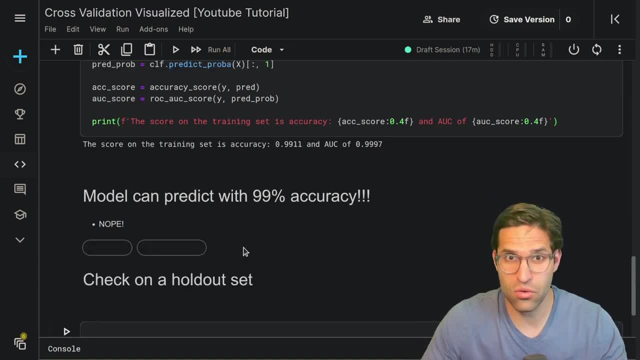 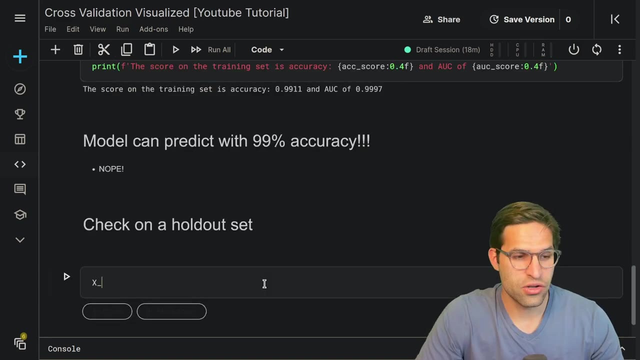 Since we did keep some of the data to the side as a holdout set And we're Pretending like that will be future data that will use our model to predict on the holdout set. We can actually score on that to see if This score is actually 99% actors. 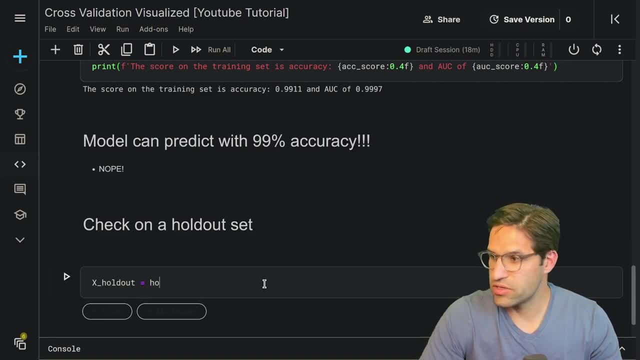 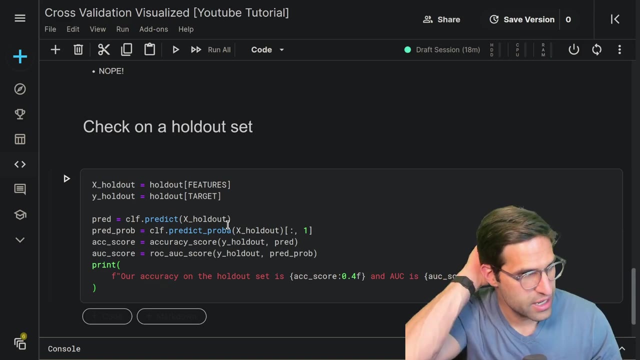 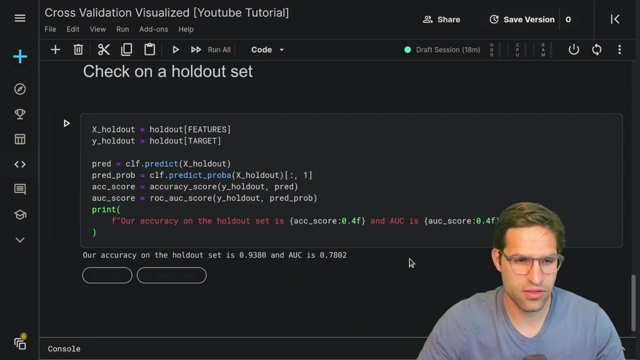 So let's make a X holdout using the holdout data features and a Y hold out- hold out target, and then we'll do all the same things we did above for predicting using our classifier, which we've trained, and scoring both the accuracy and the area under the curve score. okay, now we're back to earth here. 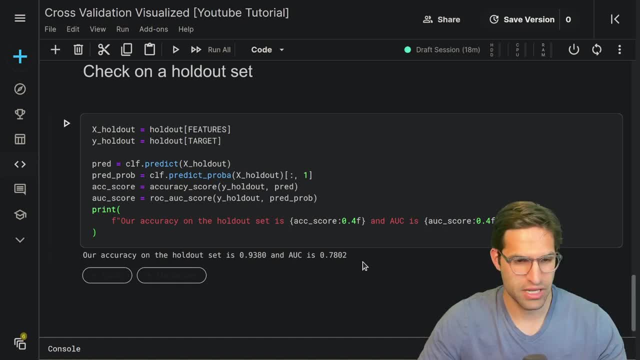 actually, if we had put this model into production and thought that we were 99 accurate, turns out it's only about 93 accurate and the area under the curve is 0.78. now, a perfect area under the curve would be 1 and a random guess would be 0.5. so this is, you know, not horrible, but if we look 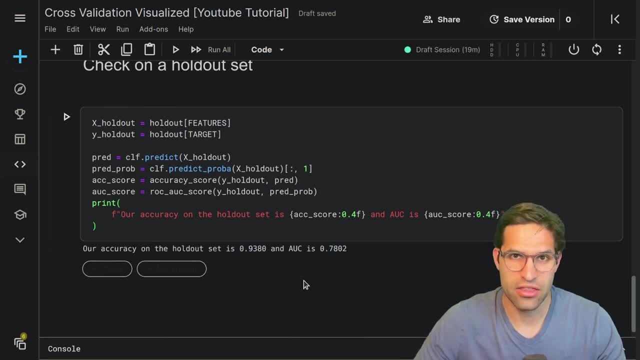 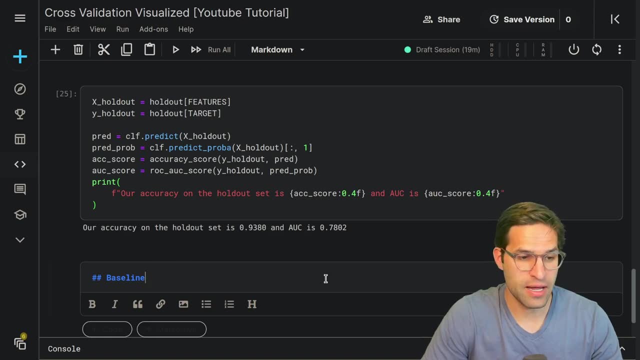 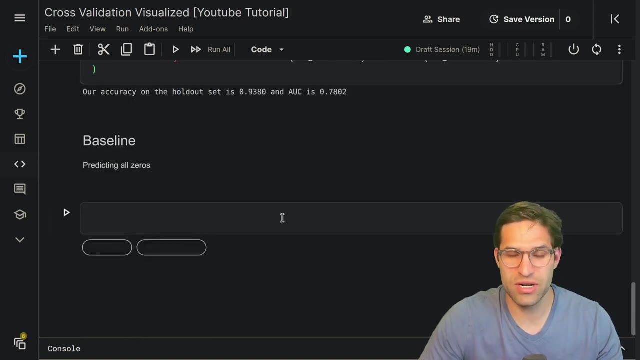 closer at this accuracy of 0.93, we might want to say: okay, how does this even compare to a baseline? let's baseline by predicting all zeros. so this is basically predicting. since we don't have an even balanced classes here, we don't have in in. 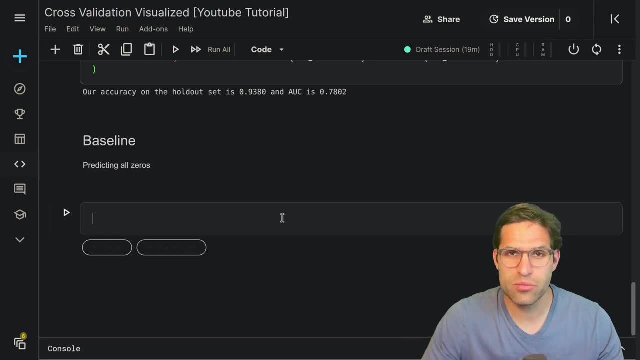 this data set is quite imbalanced. if we just predicted, everyone would not have a stroke, we'd actually get a pretty good score. so let's do that accuracy score with our target and then we'll just do numpy zeros, like, which will give us an array that's just the same shape as y, but all zeros. 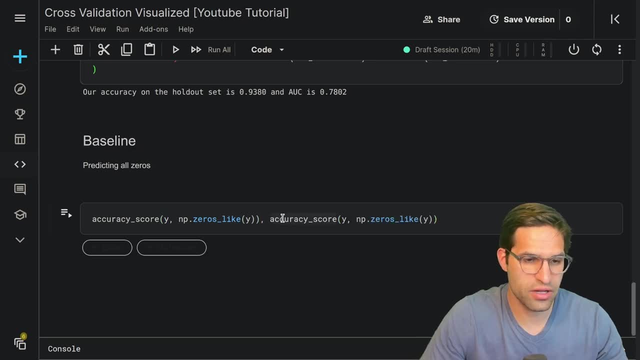 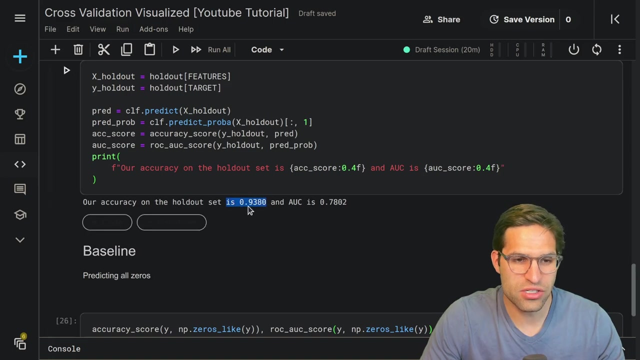 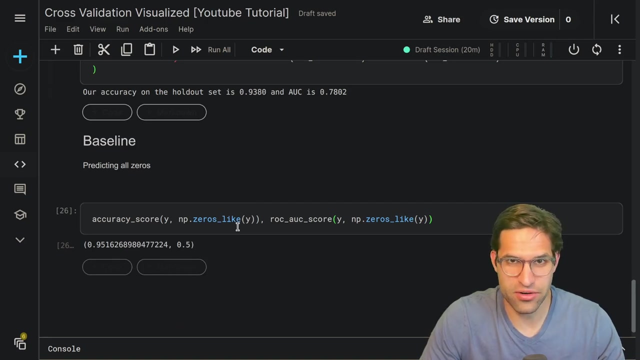 and then let's also do this with the area under the curve. so we do see here that our baseline area under the curve would have a 0.5, but actually our baseline accuracy would be 0.95. so this, this model is scoring worse on the holdout set than it would on the training set if we just guessed all zeros. 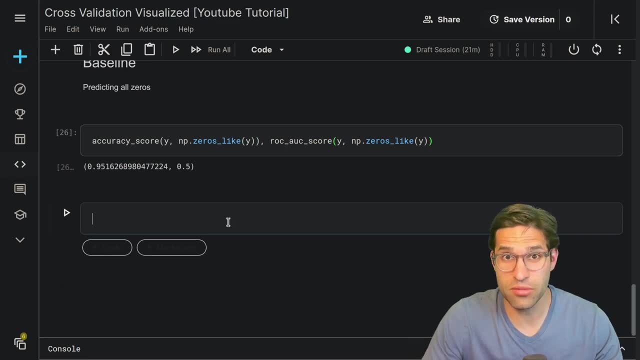 and that's not very good at all. okay, so we can see that this is a problem if we just train a model and assume that how well it does on our training data will work equally as well on any other unseen data, and the way that we can do that is: we can do this with our training data and we can do this with 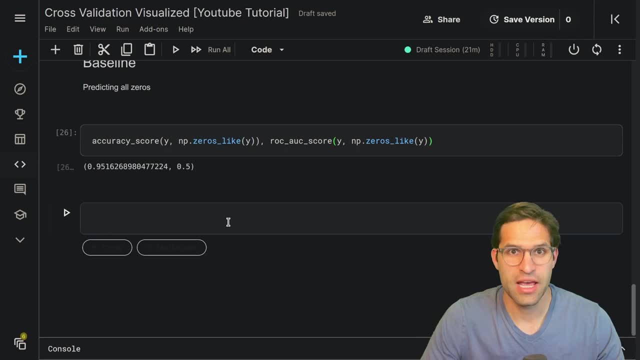 this, and we can do this with our training data. and we can do this with our training data and we can combat against this is by doing something called validation, and the easiest way to do this is just a train test split. even though it says train test, I'm actually talking about splitting our training. 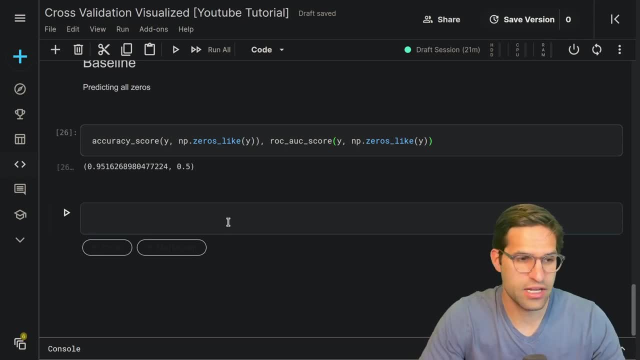 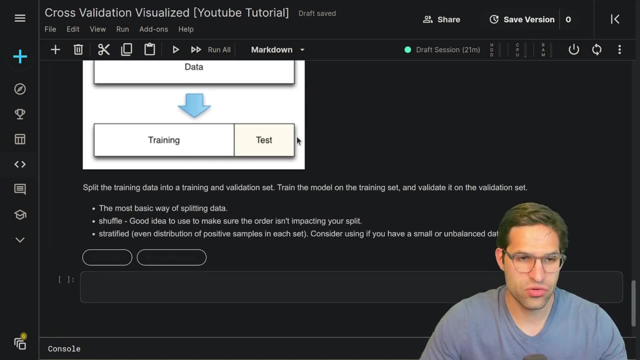 data into a training set and a validation set, and I'm going to show you how that looks here. all right, so train test split is basically taking the training data, making a training and a test or validation set, and then we can evaluate it on that validation data by using a training set, and I'm 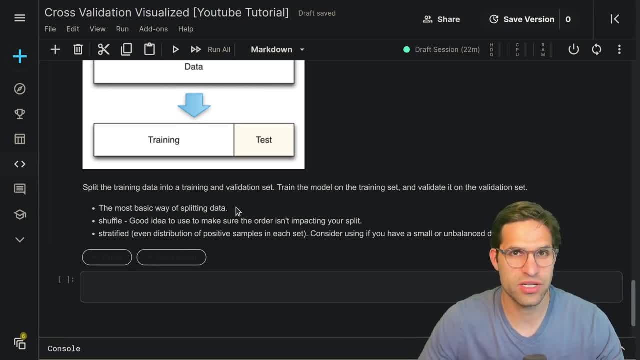 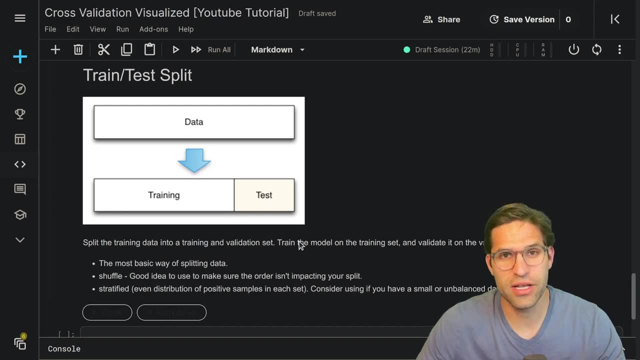 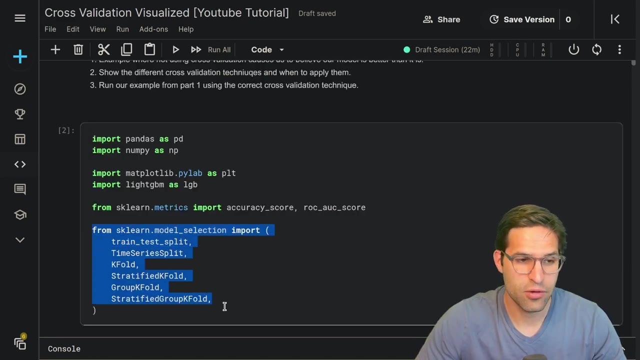 before we put it into some sort of production environment where it's going to see unseen data and we'll be able to evaluate it. This is the bare minimum that needs to be done when creating a machine learning model and trying to validate it. If you remember, before we imported train test split. 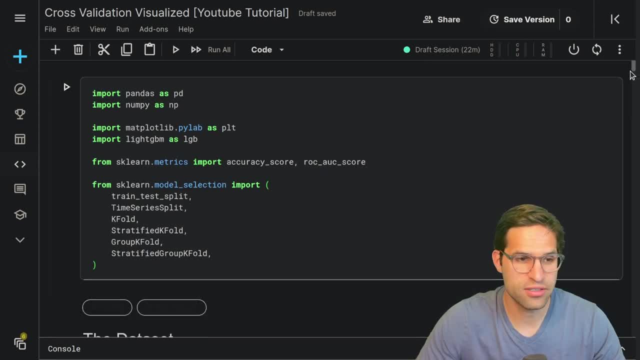 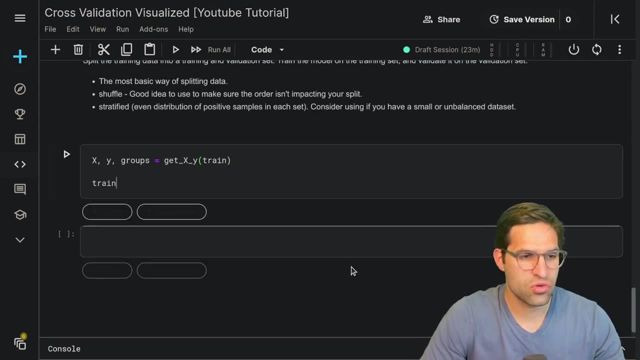 from sklearns model selection and we're gonna use that right now. First we're gonna go ahead and get our X and Y data again And then we're gonna run our train test split on this data and it'll take in a number of arrays. 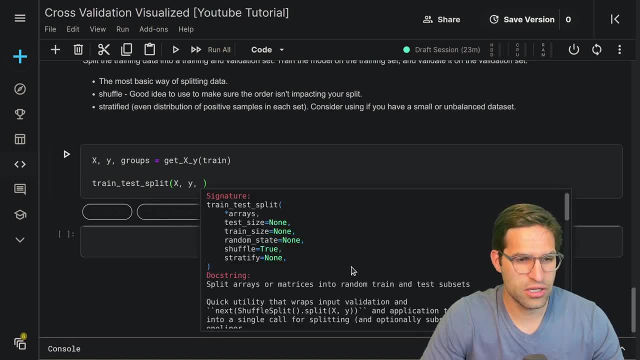 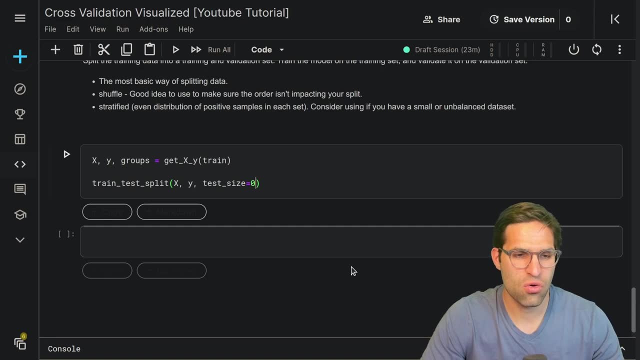 For us right now will be X and Y, and then we'll say how big we want the test size to be. We could either give it a number of samples that we want the test size to be, or we can make it a fraction. So we want our test size to be a 10th of all of our data. 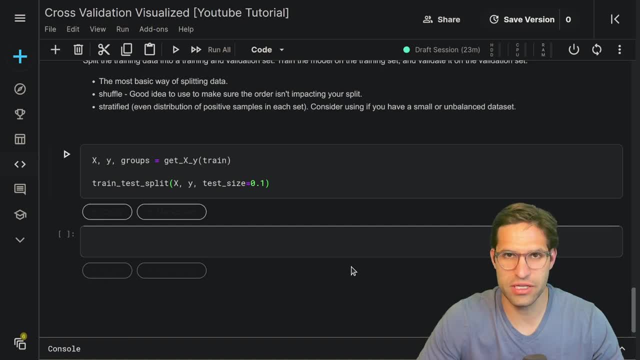 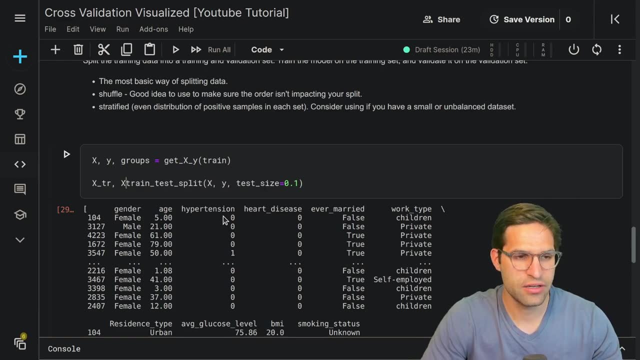 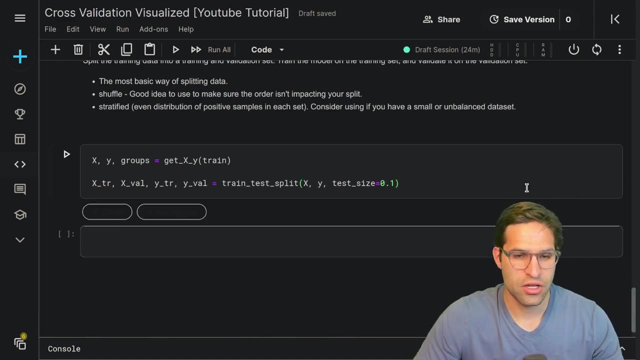 A 10th or 20% is a common split that you'll see when doing a train test split And this will actually return X train and X- we're gonna call it validation- a Y train and a Y validation. So now we can do what we did before. 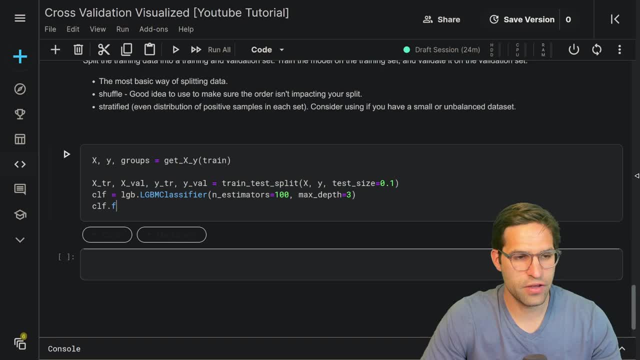 and that's creating a classifier. We can fit our classifier on an X train data and then we're gonna predict on our validation data and we'll do the predict probability as well. We'll do the predict probability as well. We'll do the predict probability as well. 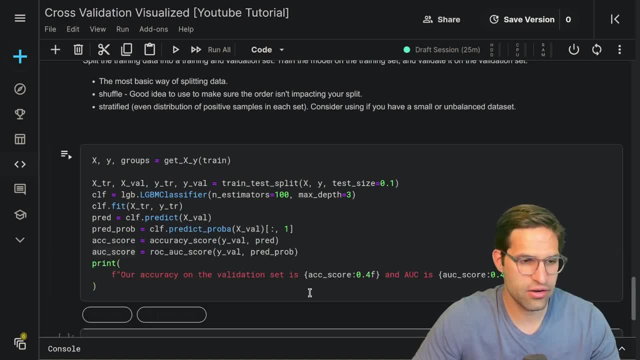 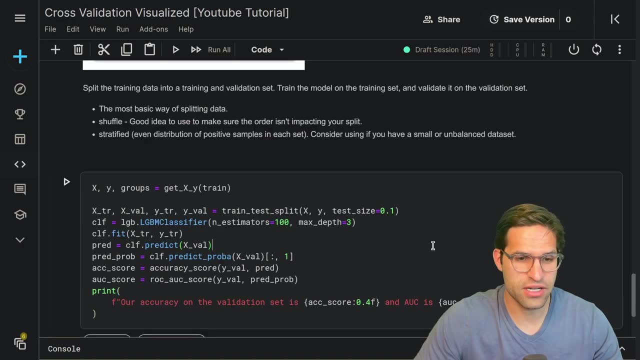 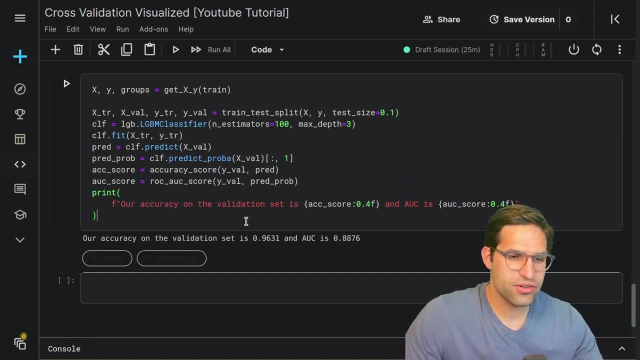 Let's go ahead and score the accuracy and the area under the curve for this model that was trained on our train split on this validation holdout split. Now we can see that our area under the curve and our validation accuracy are more reasonable and more in line with what we might expect to see. 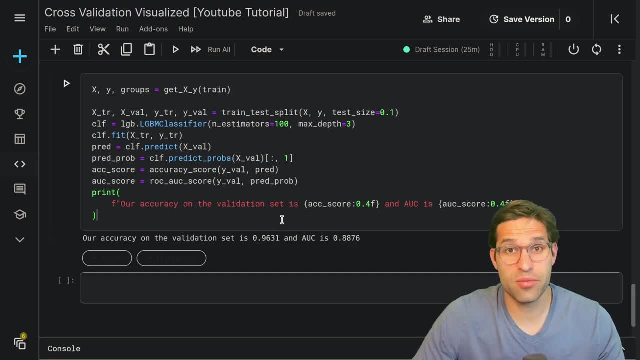 on our holdout set or our future data. This is a better representation of how good our machine learning model is- of how good our machine learning model is, But it also leads us to the possibility of fitting parameters and choosing a model that's over fit to this split. 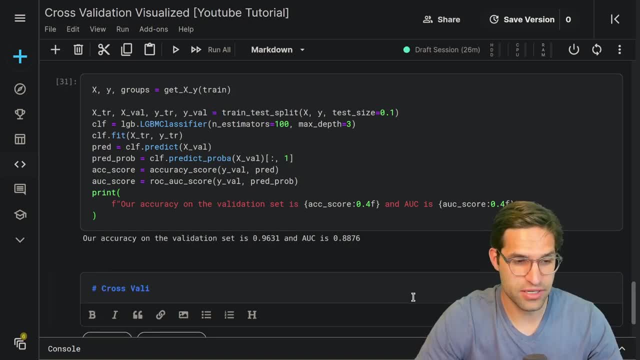 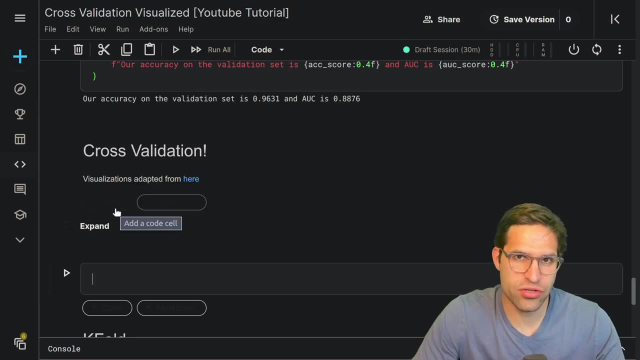 And that is where cross-validation comes in. Okay, so we're ready to talk about cross-validation and why it's so awesome. Now I'm creating some visualizations here to help us visualize what's going on, And most of it's adapted from the sklearn library documentation itself. 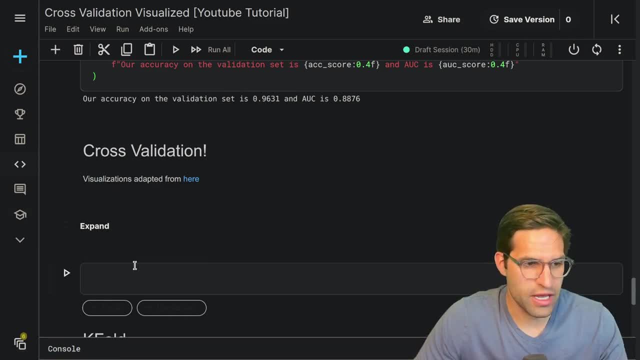 I don't want to get bogged down in all this code itself, So I've hidden it, But the basically what you need to know is I've created a function called get fake xy, which allow us to get xy in groups, just like before, but just for some fake data. 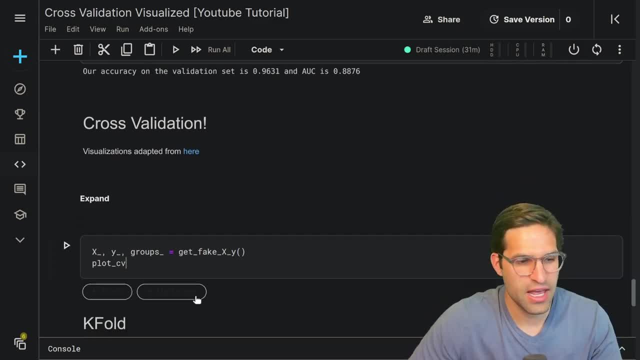 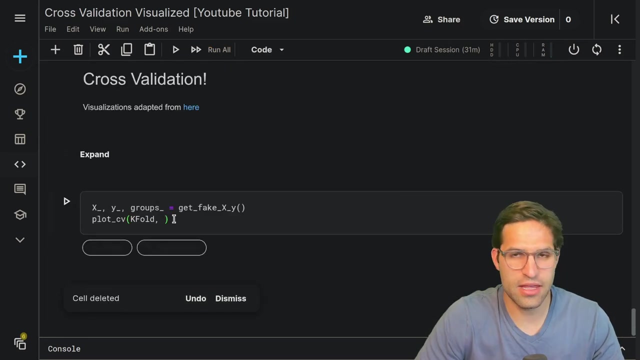 that'll be cleaner to for evaluating in this plot. And then we have a plot CV function And what this takes is a different cross-validation technique from sklearn's library. So we're going to put in k-fold, which will be our first example to show. 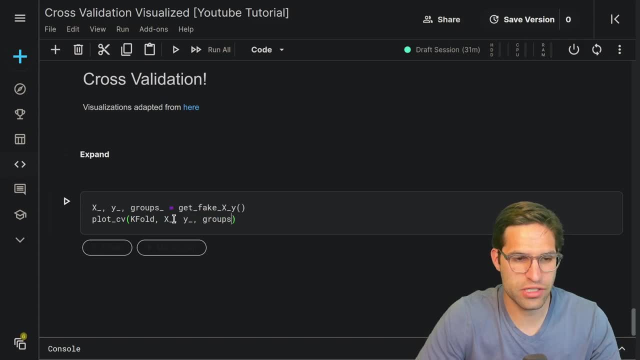 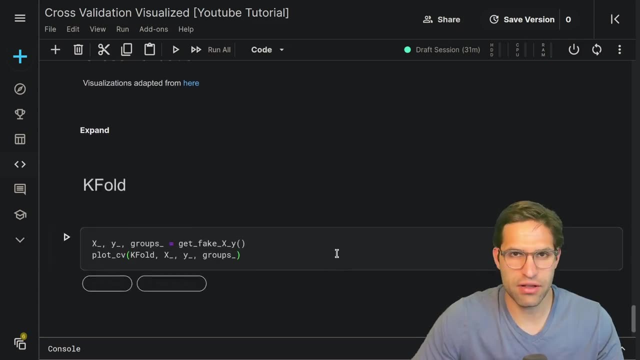 And then we will give it our data and it's going to make a pretty visualization for us. So yeah, we're going to first talk about k-fold. This is a very common cross-validation technique And essentially all it is is taking our training data. 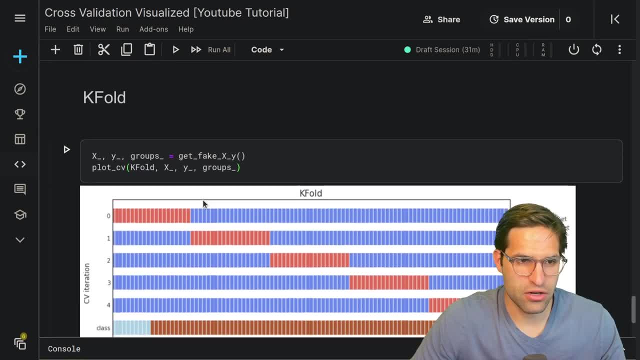 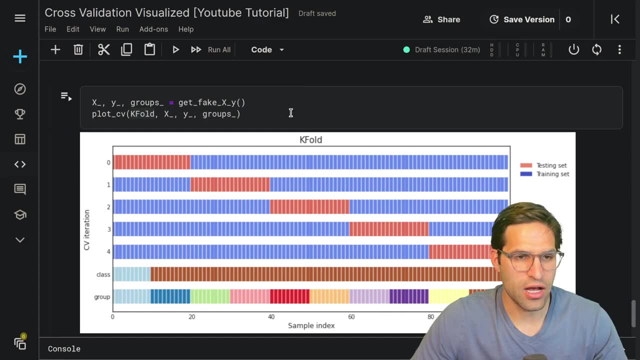 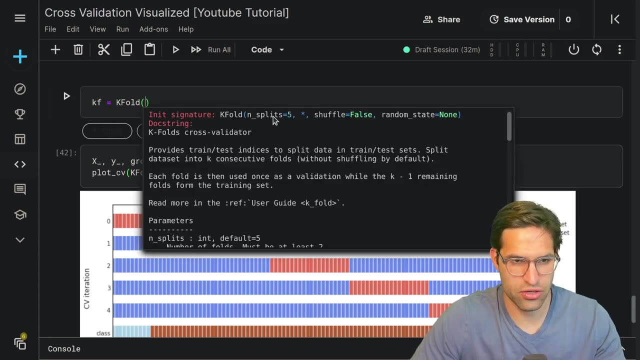 and splitting it up into different groups. By default, it'll just split it up evenly into chunks, depending on the number of splits that you give it. So let's create a k-fold object here with k-fold and show you that you can set the number of splits. 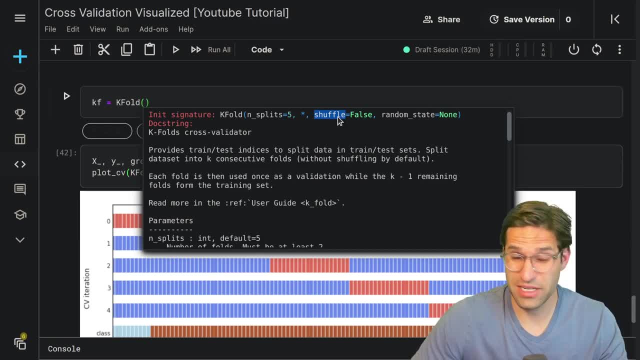 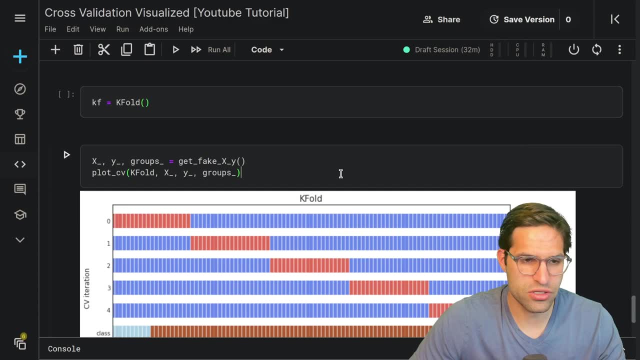 You can also set it to shuffle or not. It's always a good idea to shuffle it if you're not sure, And then you can set a random state for the shuffling so that you can recreate the same results in the future if you would like to. 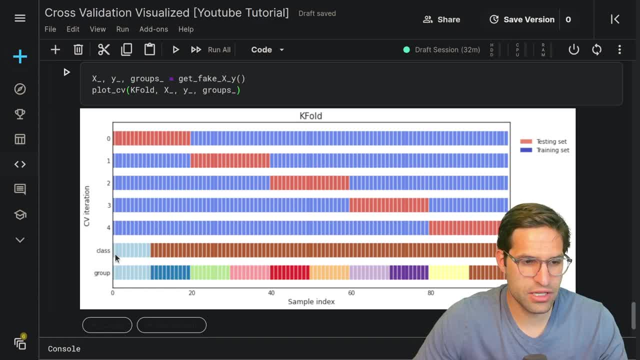 But this visualization shows us how this looks. So imagine the class here being the ones or zeros We're predicting likely or not for their stroke, And then the group here would be our doctor column, where we have different doctors who have gathered this information. 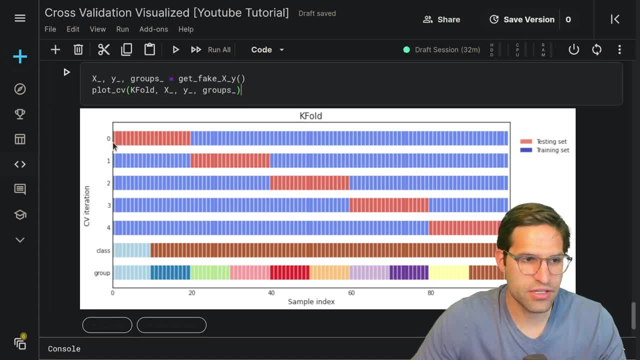 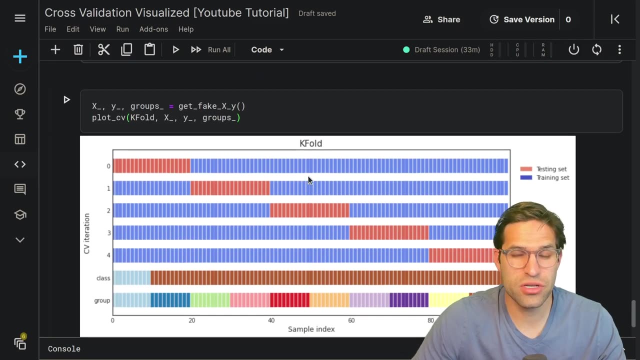 Now, k-fold splitting basically gives us however many splits. So here we have five where we've split the training data into a training and a testing set or training and validation set, And we've done that five different times. So you can already see why this would be even more powerful. 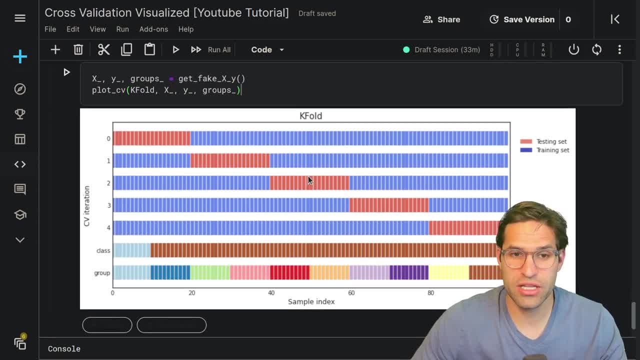 than the train test split. We're essentially doing this with all of our training data and we're evaluating five experiments instead of just zero. Now you can make the splits more or less. Five is a pretty typical number, but the more splits that you have. 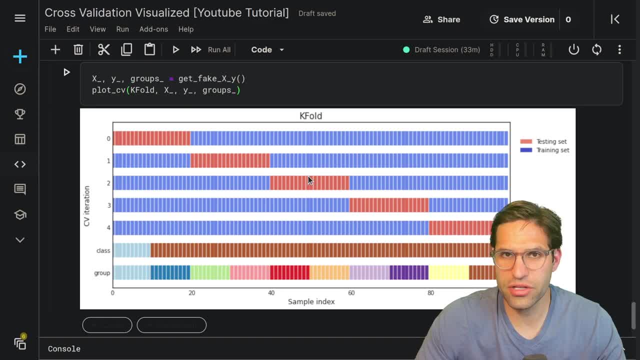 the longer your training time will be, And there are other things you might want to consider, like if you split it too small, then your test set might not work. You might not actually have enough test samples to be predictive or to show you how well your model is doing. 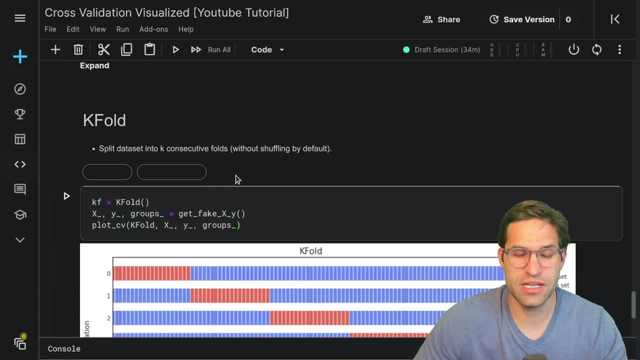 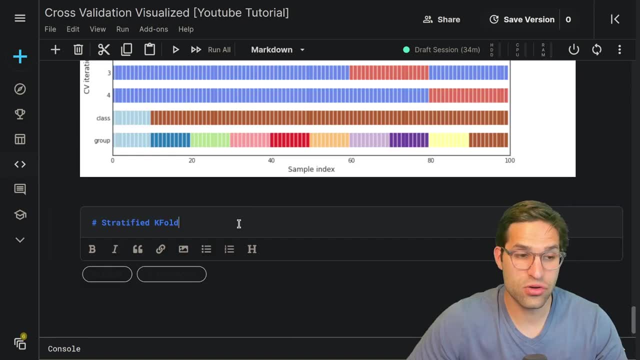 So basically k-fold, it splits our data set into k consecutive folds without shuffling by default, but you can set shuffling as true. The next cross-validation technique is called stratified k-fold And it's very similar to the k-fold from above. 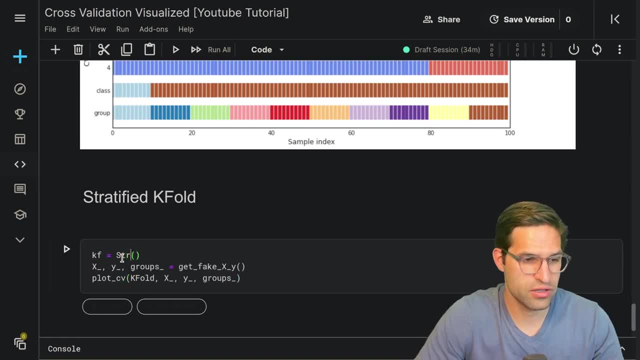 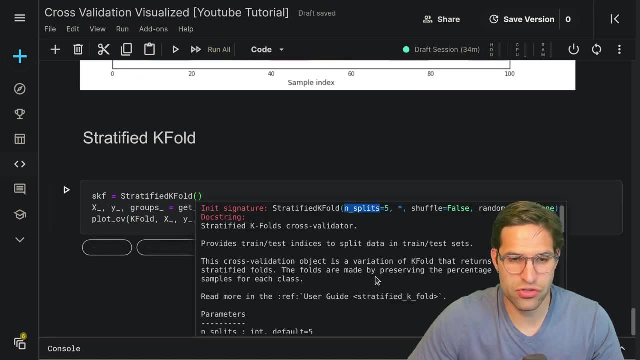 but we're going to show how this works. So stratified k-fold, Let's call it s-fold, S-K-F, And, just to show you, you can also choose the number of splits, whether to shuffle or not, in the random state. 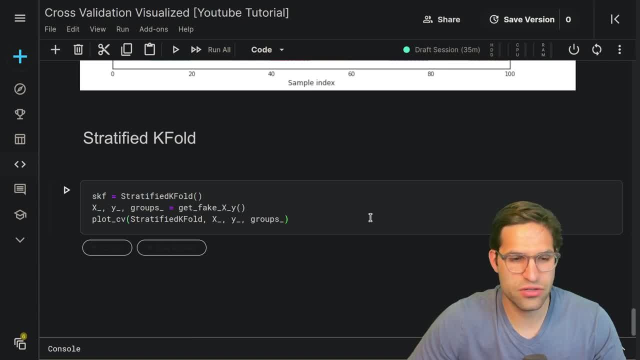 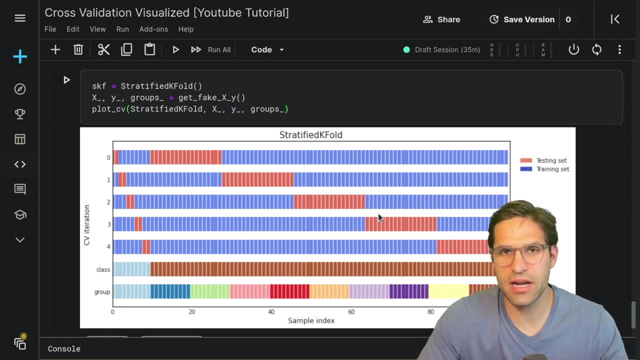 And let's pass this through our visualization tool to see how the splits look Now. the difference here is: stratified k-fold will automatically try to balance your target variable in both the training and the validation set, And this is important, especially if you have an imbalanced data set. 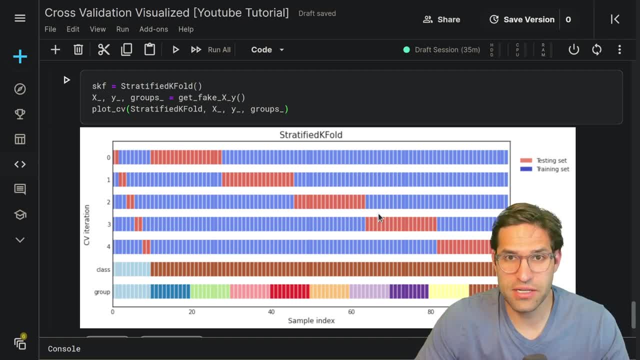 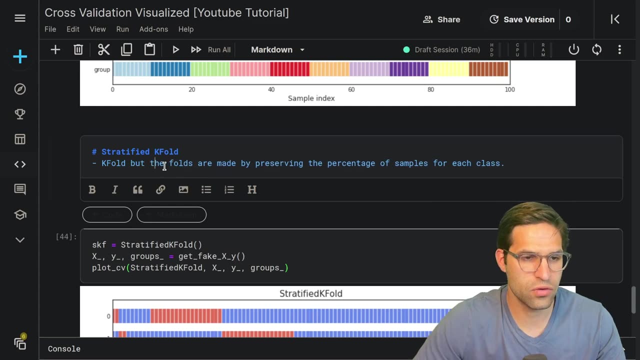 where there's a chance that you might have no positive cases in the validation set if you let it up to chance. Stratified just makes sure that they're equally balanced groups and it's pretty common to use. So this is k-fold, but the folds are made preserving. 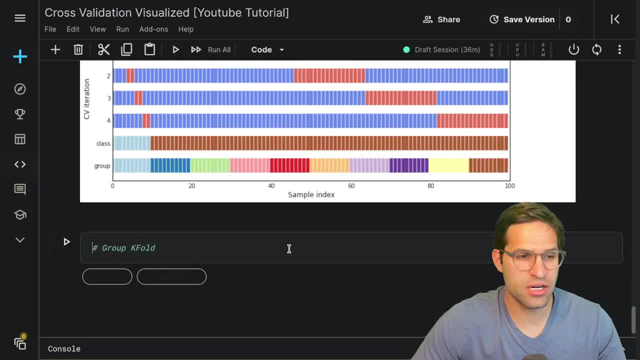 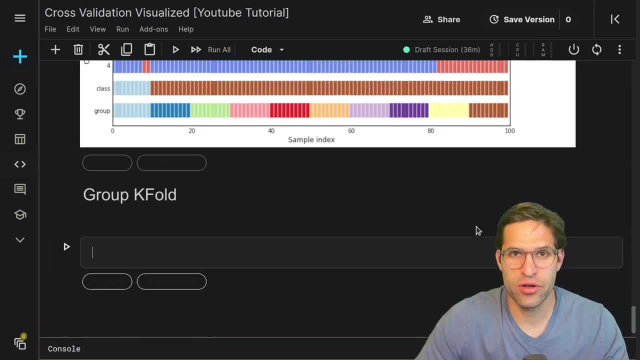 the percentage of samples in each class. Now, next we're going to talk about something called group k-fold. Group k-fold is very similar to the other two cases we showed, but that counts for if your data has some sort of grouping in which the data was gathered. 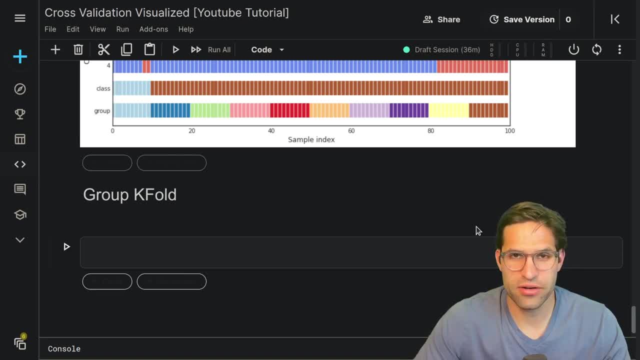 or the way samples are associated with each other. So in our case we have a doctor who may have its own biases in how the doctor collects the data that we're trying to model, And we want to make sure that our model is robust enough. 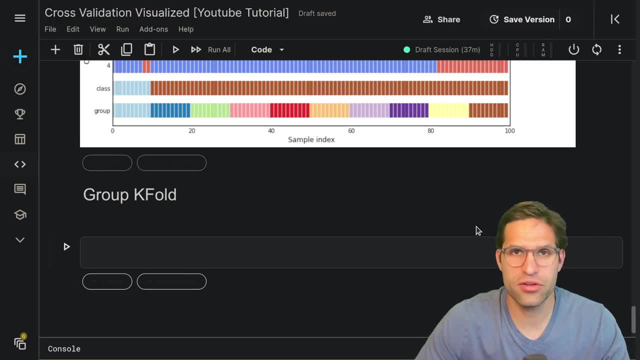 to predict well on unseen data in a brand new doctor. So by using group k-fold we can ensure that our model is validated on a different group than it is trained on and that there's no leakage or information about the doctor itself that the model is learning. 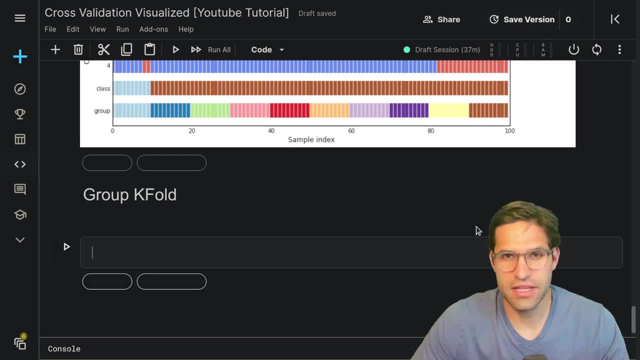 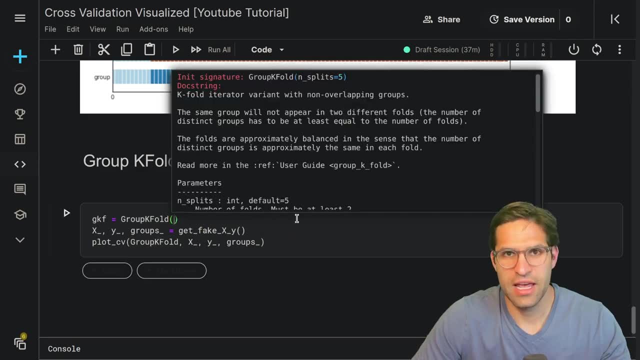 and showing our results to be more confident than it actually is. So I'm going to make a group k-fold object here and show you that in group k-fold you don't have an opportunity to shuffle or splits, It's just going to choose the same group k-fold. 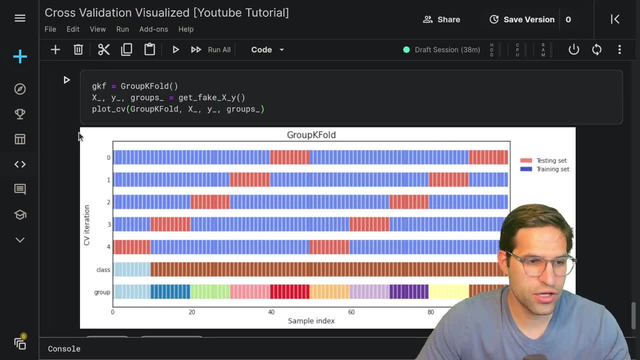 for you each time, And you can see here that for each of these cross-validation iterations or folds, you have an entire group staying together in either the train or the test set. Another example of this might be if you have a bunch of different observations. 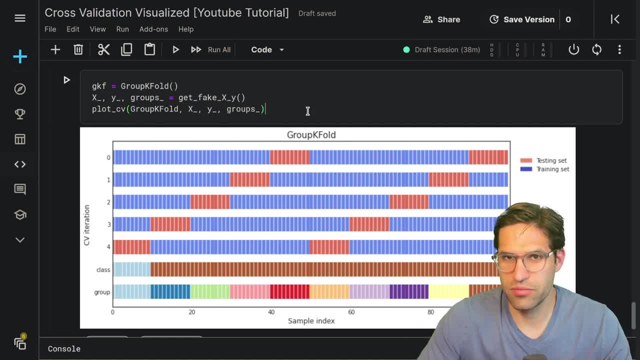 for the same person. you wouldn't want that person to be in both your train and validation set, because your model might just predict that person very well. So it is very important to consider things like group k-fold when you have data that might have information. 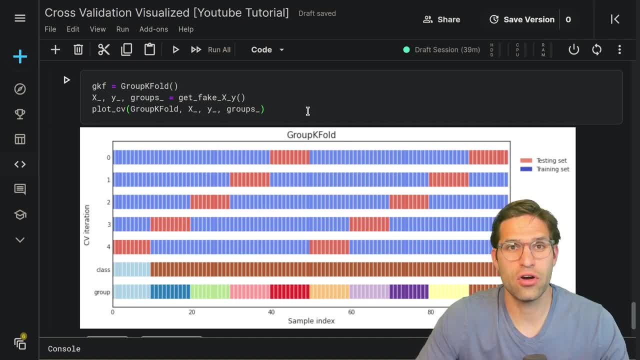 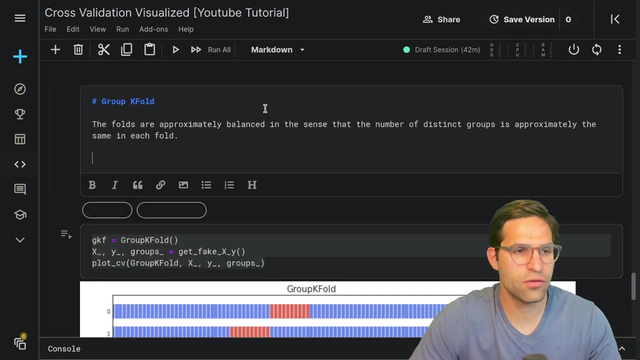 spread across different observations that could make your validation overconfident in how well it's predicting. In reality, it's just able to predict those groups, which isn't very helpful on future data where those groups might not exist. So in group k-fold. 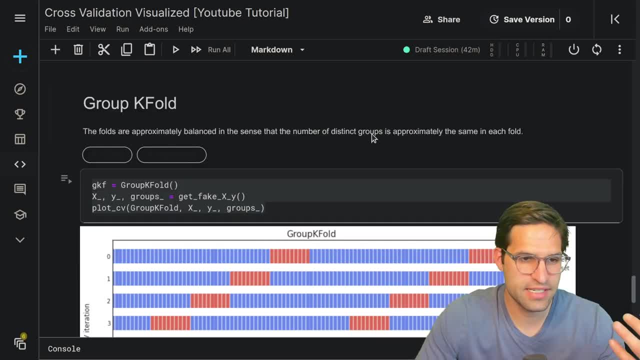 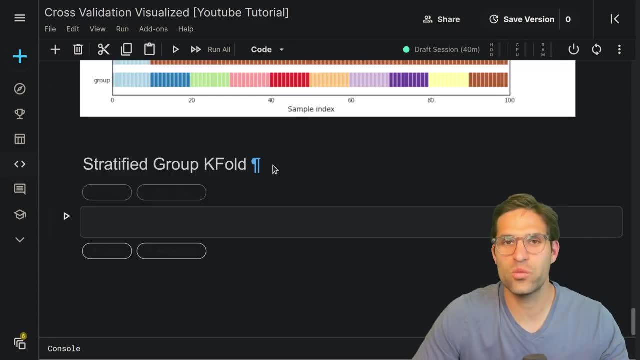 we have the folds are approximately balanced, in this sense that the number of distinct groups is approximately the same in each fold. All right, so next up, we have stratified group k-fold, And if you're tracking with me so far, you probably have an idea. 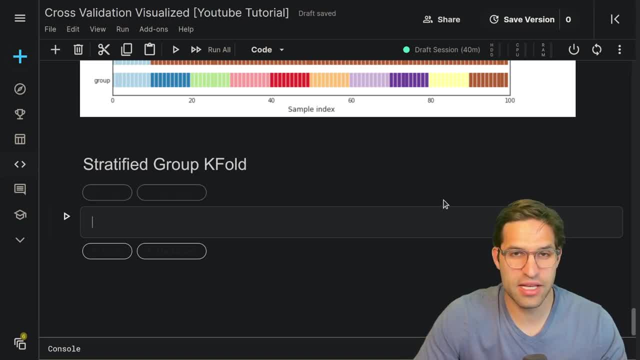 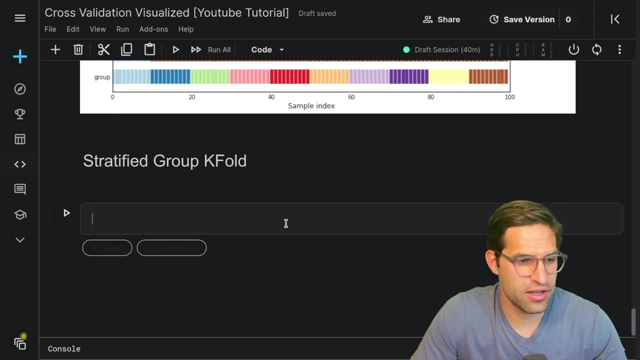 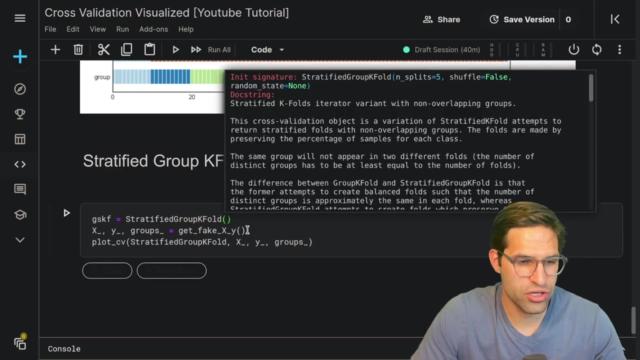 of what stratified group k-fold is. It's the same thing as the group k-fold, but ensuring the equal number of positive cases in each group. So if I paste this here- stratified group k-fold- I can show you that when you create this object. 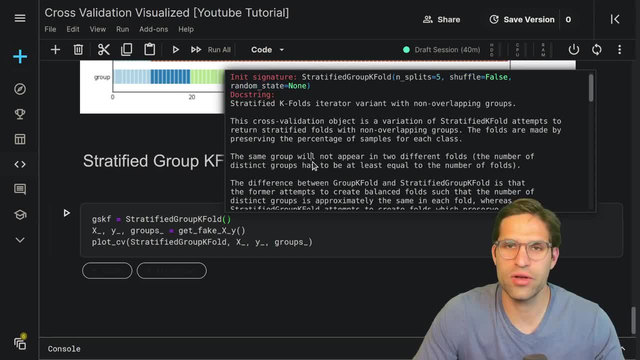 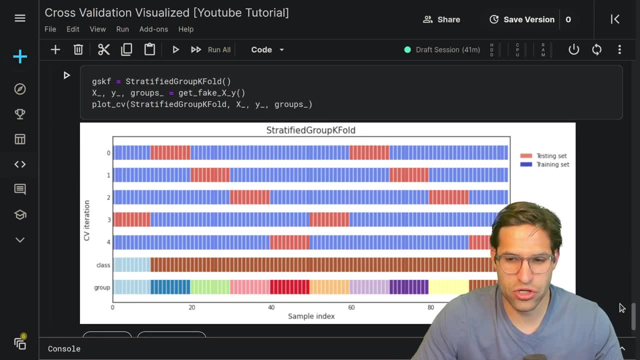 you can put the number of splits, shuffle true or false, and then the random state And to visualize it here, you can see, now that the groups are chosen, the training and test or validation set is split so that the groups are preserved. 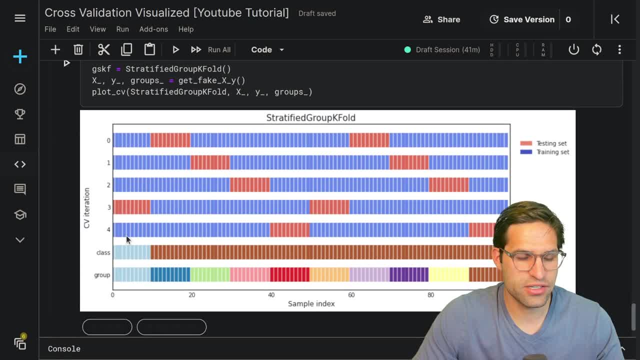 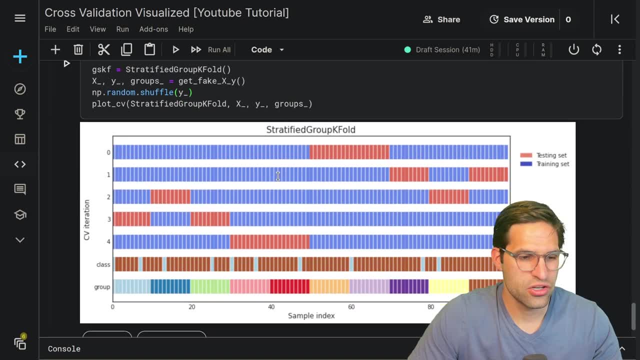 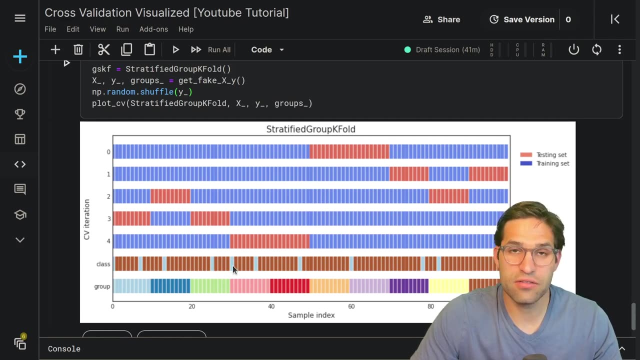 but the groups are chosen such that there's an even distribution of the class in each of these samples. If I shuffle the target class, you'll actually see it a little bit clearer, because the groups for our target class might have different amounts of targets and it'll choose the right amount of splits. 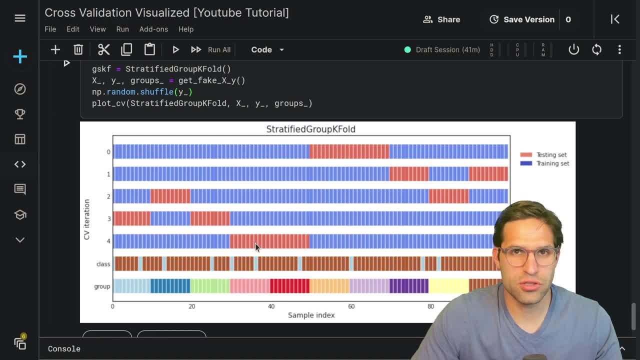 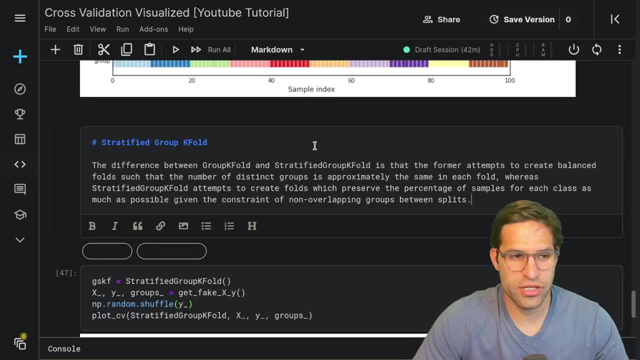 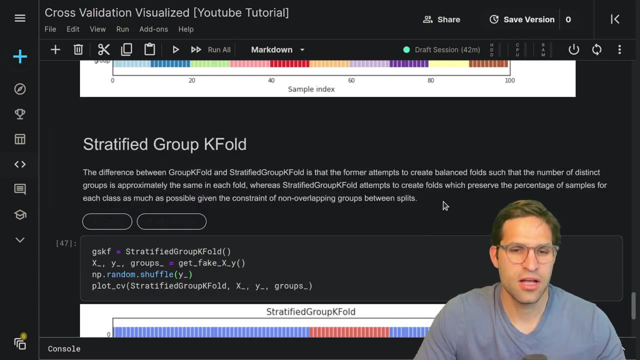 so that you can have multiple models created across folds and get a balanced split of your target variable. And if I show you the description from sklearns library about stratified group k-fold, it goes into a little bit more detail but essentially 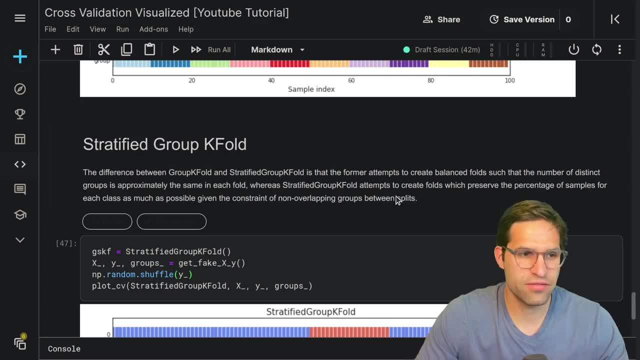 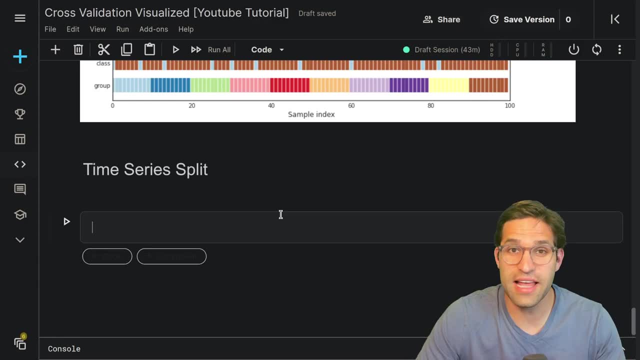 it's trying to preserve the percentage of samples in each class as much as possible, while preserving the non-overlapping groups. Now, the last type of validation technique I want to talk about isn't really applicable to this data set, but it is very important if you're using any sort of time series data. 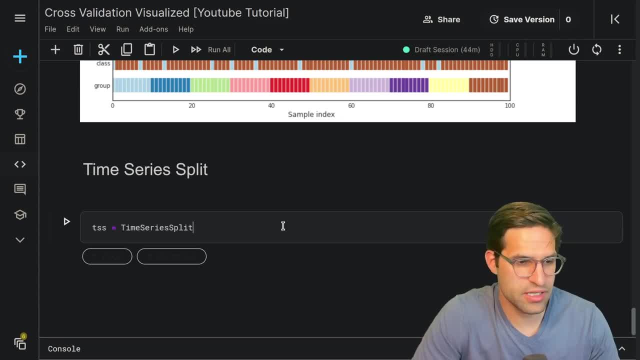 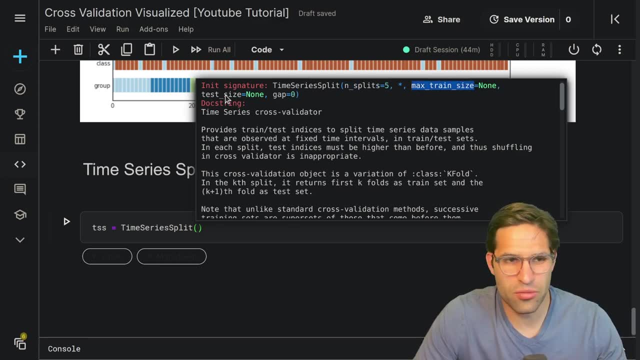 and that's called the time series split. So let's make a time series split object and just show you You can also have the number of splits, just like the other one. Then you have some other parameters like the max train size and test size. 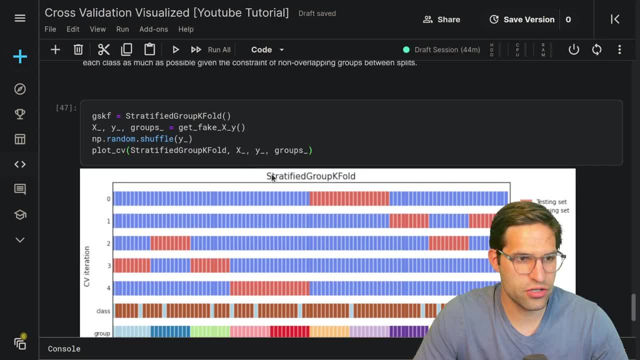 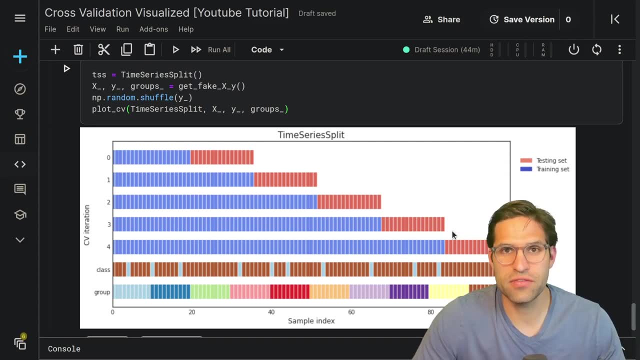 and a gap. This will become clear when we actually visualize it. So in a time series split, you want to make sure that none of the information about the future is fed into your model, to give it observations about something it shouldn't have seen at that moment in time. 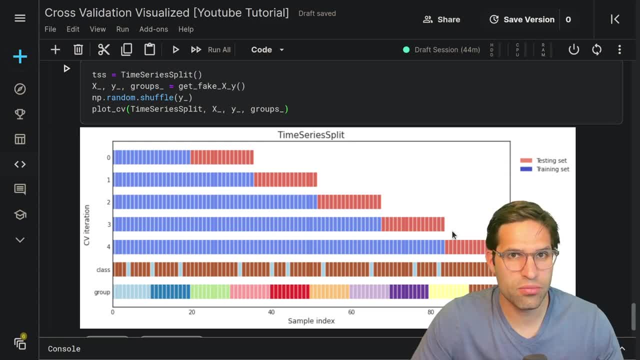 So it also is known as a sliding window approach, where you grow the amount of training data that you're providing it in time and then testing on the amount of time right after the training period ends. If I do a video on time series machine learning. 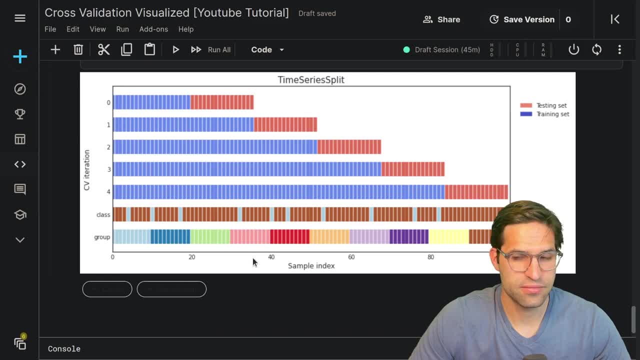 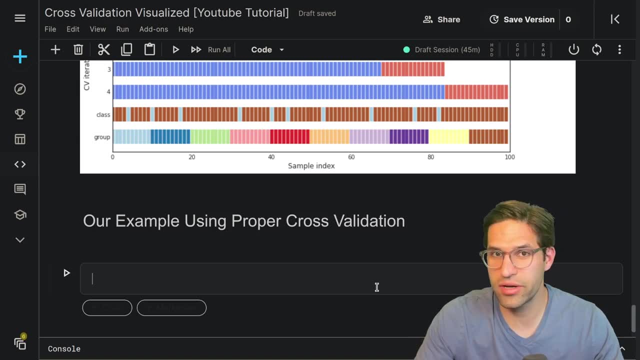 I will make sure that I cover this in detail. Okay, now that we've learned about some of the cross-validation techniques, let's go back to that first example and try to recreate what we did, but with a proper cross-validation technique. So we know we have a small data set. 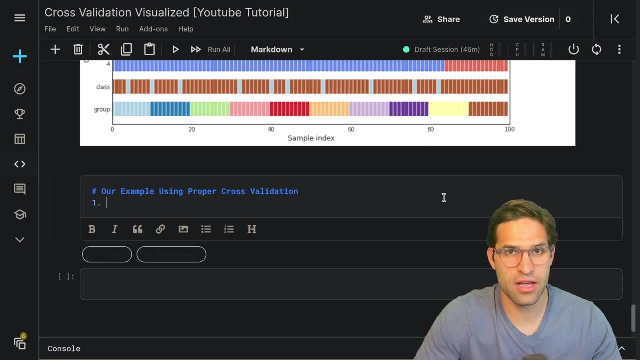 that's very imbalanced. So we want to make sure that we have a balanced number of samples in our validation set that are true. It means we're going to use stratified. We also know we have some sort of grouping, like the doctor information. 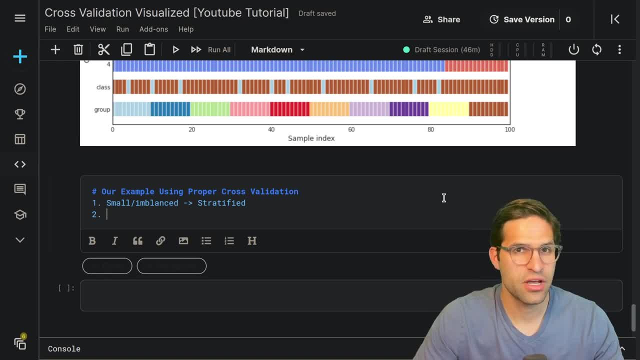 where some of the samples come from certain doctors. We want to make sure the same doctor's observations are not split between the training and validation set, So we're going to use a group validation technique. So in this case I would use a stratified group k-fold split. 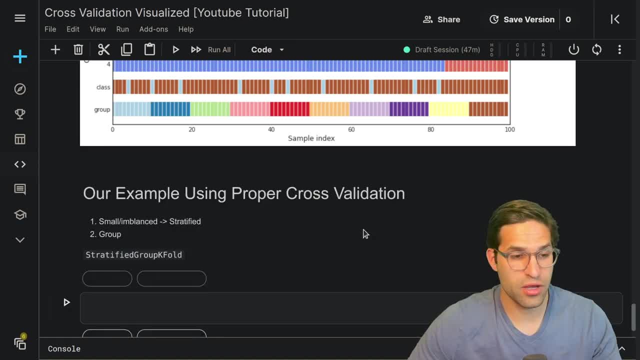 We're going to set up it with number of splits equal to five. We're going to also make sure that shuffle is on, to make sure that the sorting of our data doesn't play any role into how the splits are made. So let's go ahead and create. 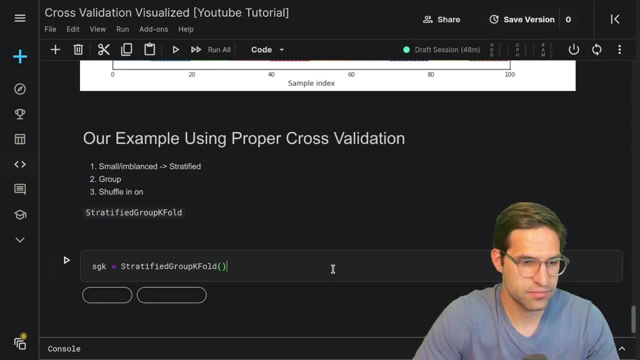 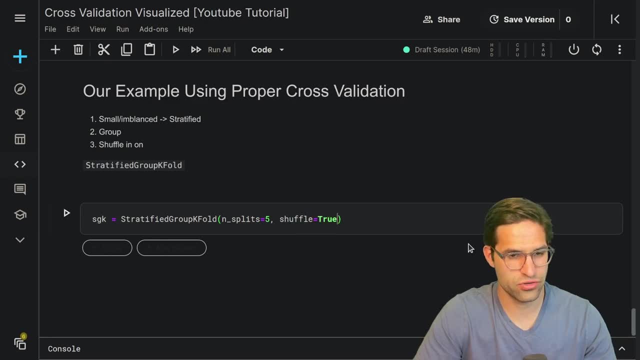 this stratified group k-fold object: We're going to give it the number of splits, which is five. We're also going to put shuffle as true And let's go ahead and give it a random state, just so that the shuffling is the same. 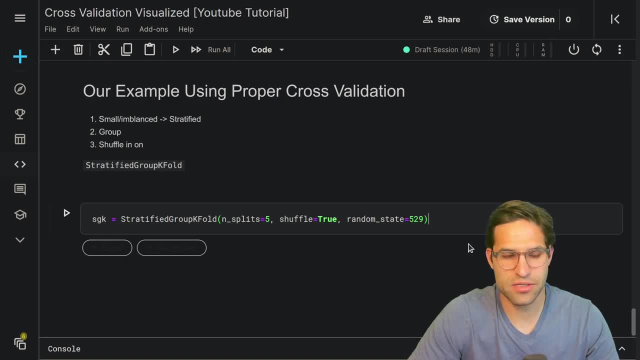 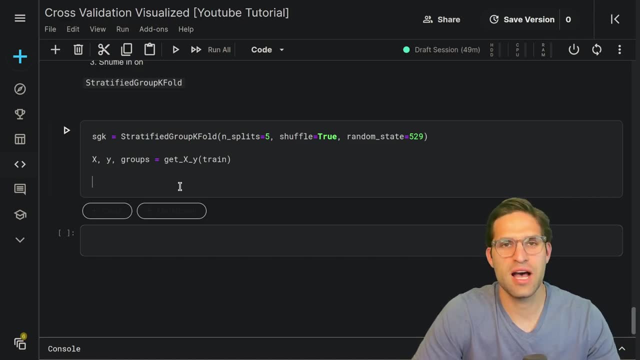 every time we run an experiment, so we compare apples to apples. Let's go ahead and run our get data again. So now that we have our group stratified, k-fold object, we can run the split method on our data like this: x, y, we provided our groups. 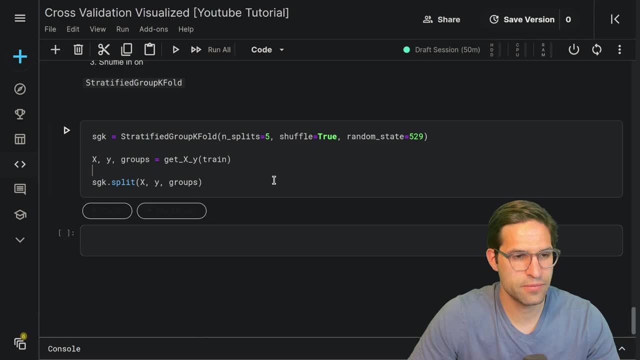 You can see that the split method takes x- y in the groups. So if we run it, we can see that this object is a generator and it runs these splits, and it'll provide us, every time we iterate over it, training and validation indices. 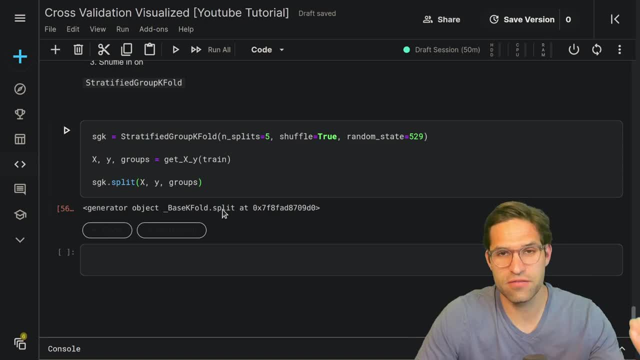 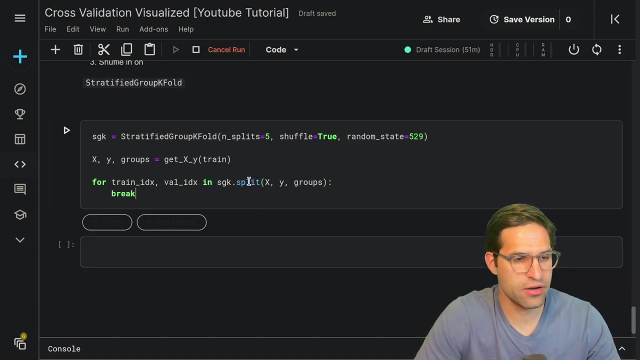 So the locations where the train and test value samples should be taken from. So we can loop over this by saying for train index and val index in this generator. And if I break here, I can just show you that the train index are just numbers of where in our training data set. 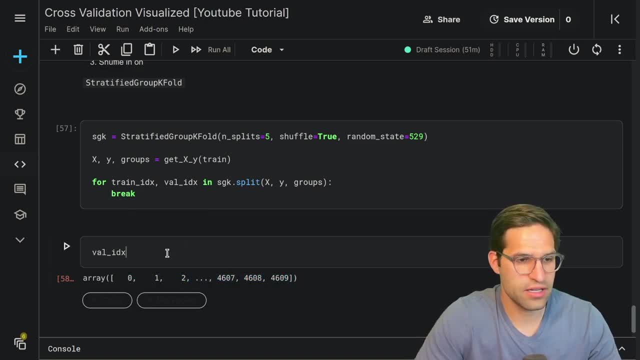 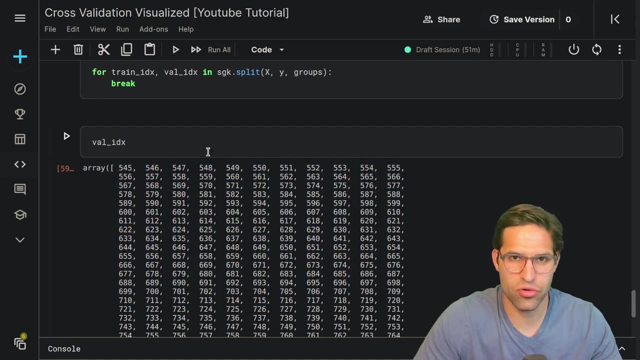 we should pull out the training samples And the val index are the samples that we should be using as validation, because we're using group k-fold. They'll all be in the same group. That's why you see these numbers starting at 500.. 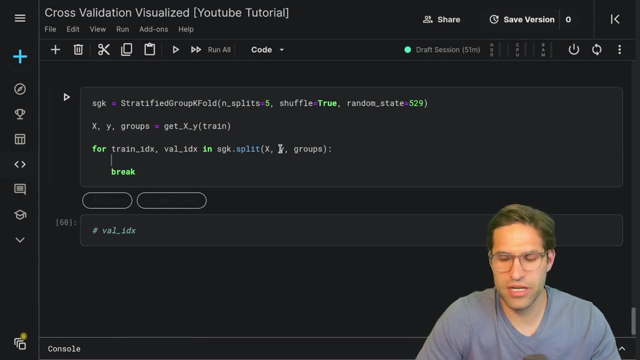 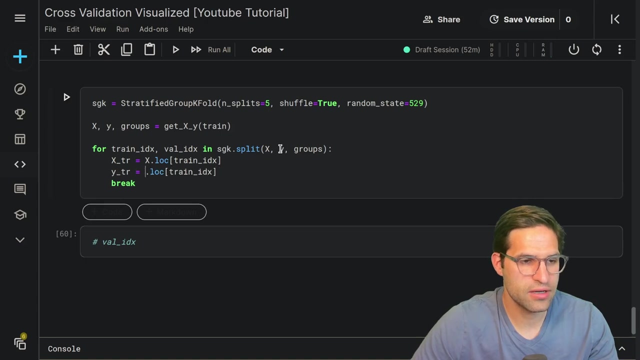 And now we can- similar to what we did before with train test. split is we can run the train, We can pull out these samples and create a train and validation. So let's locate in x, where the train index appears. We'll do the same thing with y. 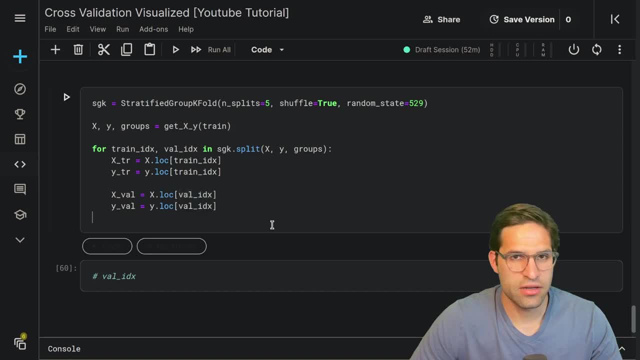 And then we'll do this for our validation, val index. Now, there's a lot of things we can do at this point, like saving the fold number into our data set or saving out of fold predictions. That's beyond the scope of this video. 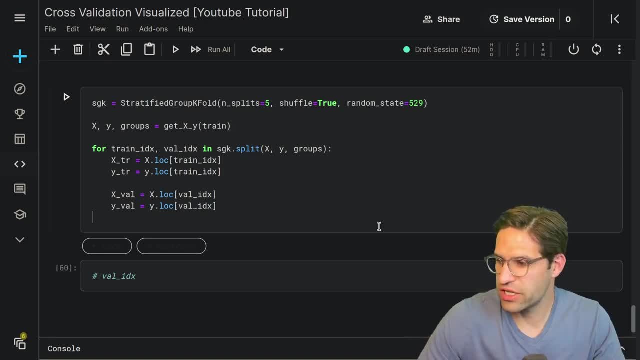 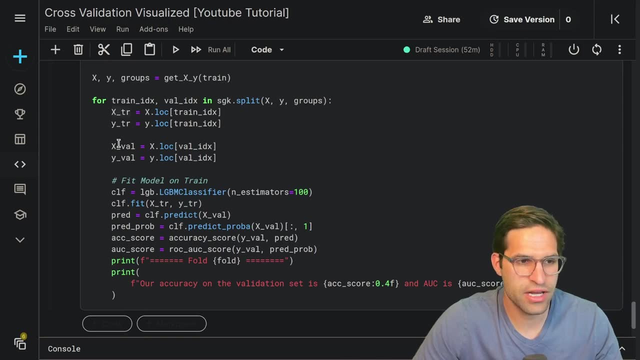 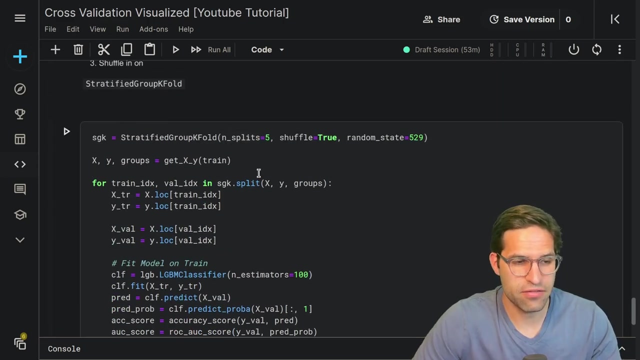 But just to show how this works, we're actually going to do the fitting and predicting like we did before. This just runs the fitting of the classifier on this training set and validation set And this will loop over five different times because we set the number splits to five. 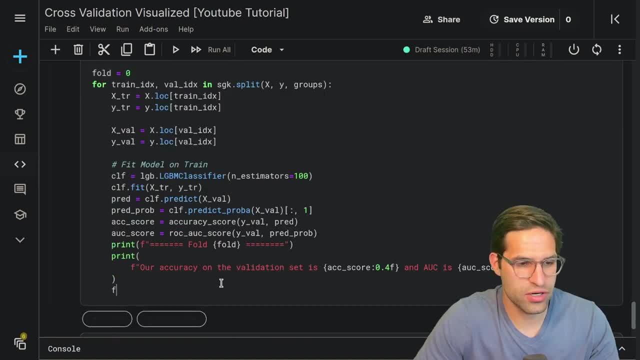 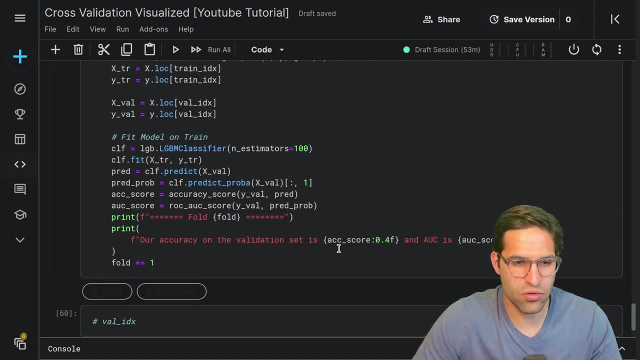 Let's actually name each fold And then at the end here we're going to do a fold plus one, So it increments each time, And we'll print out our scores for each fold, similar to like what we did before. There we go. 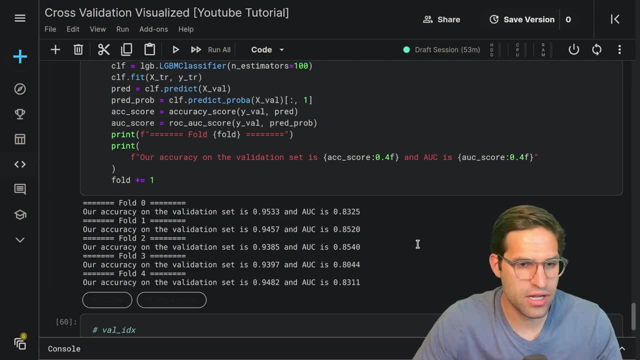 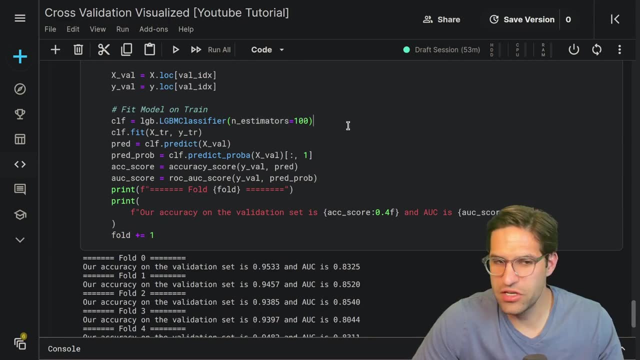 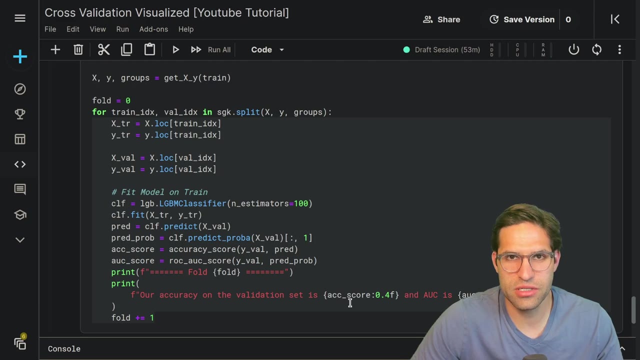 So we have a more robust way of evaluating this model setup. Anytime we change any parameters to this model or we're changing the features we create in the model, we would want to do it within each cross-validation fold, So within each of these loops. 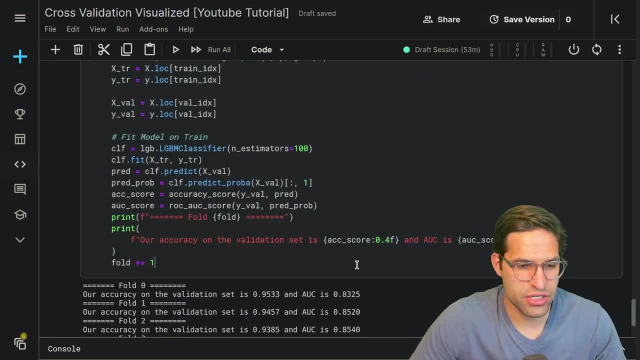 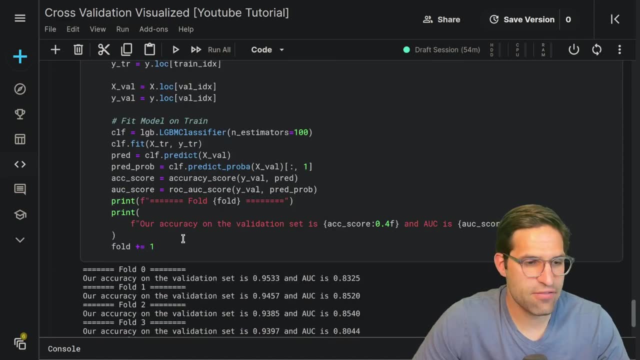 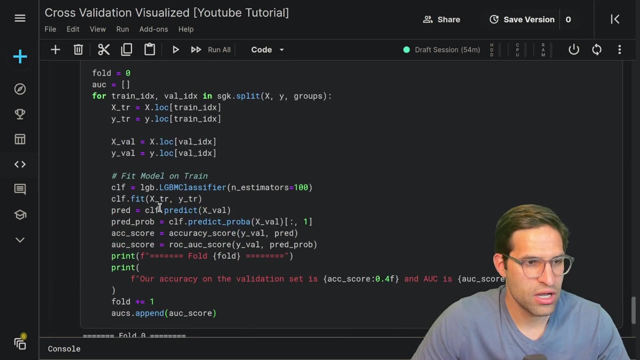 to really fully get the best out of this cross-validation scheme. Additionally, we can save off the scores that we have for each fold and then average across them to get a more robust idea of what our area under the curve score will be. So creating a list here for AUCs to be stored.